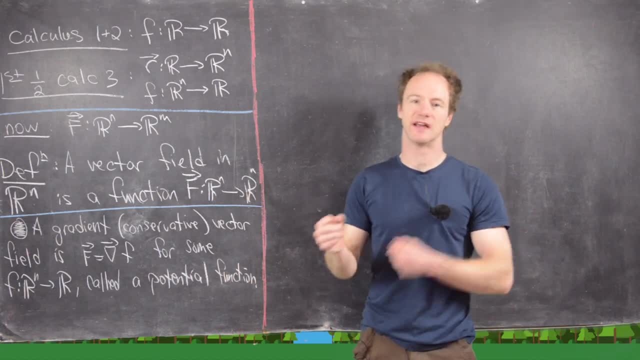 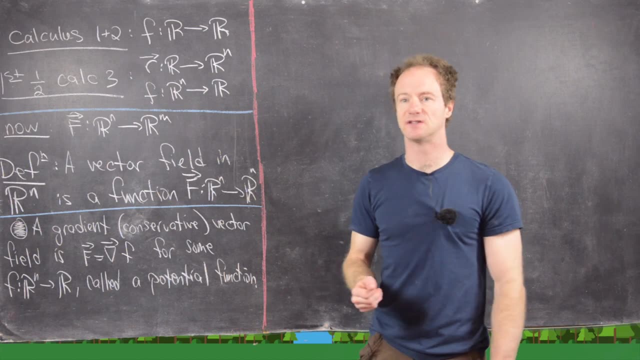 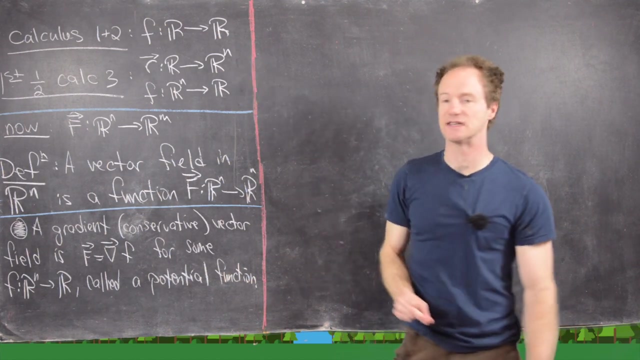 So remember, we had partial derivatives, we had multiple integrals and so on and so forth, And generally here we wrote things like z equals f of x, y, or maybe like w equals f of x, y, z. Okay, so now we want to generalize this by putting these two ideas together. 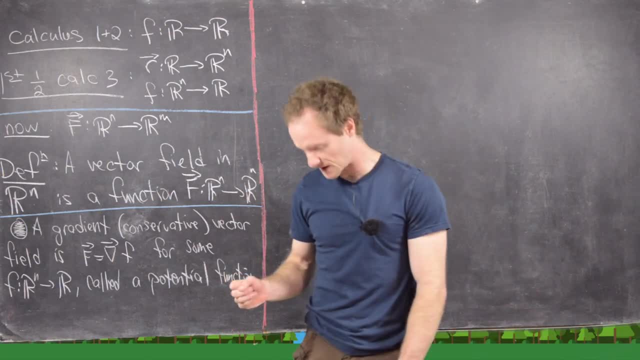 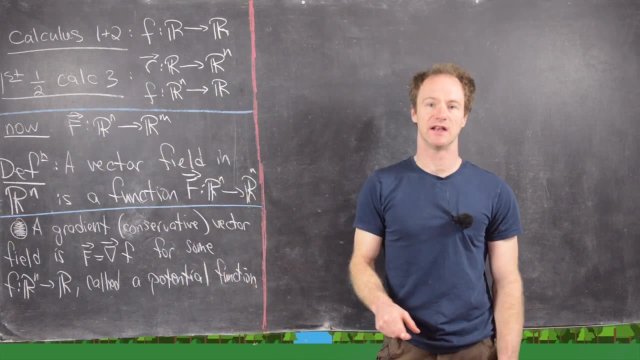 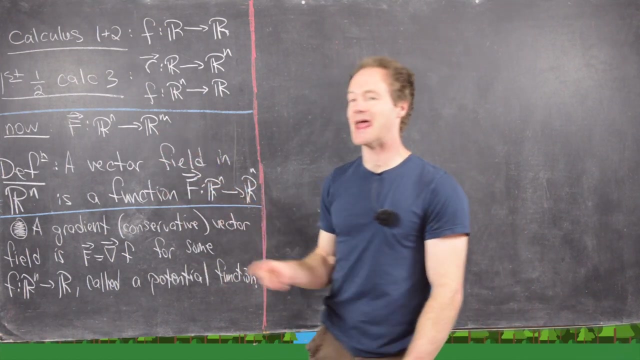 And so the most general way to do that- which is something we won't do- will be: we have a function whose domain takes n inputs in. In other words, it's an n vector and its codomain or its range gives us an m vector. 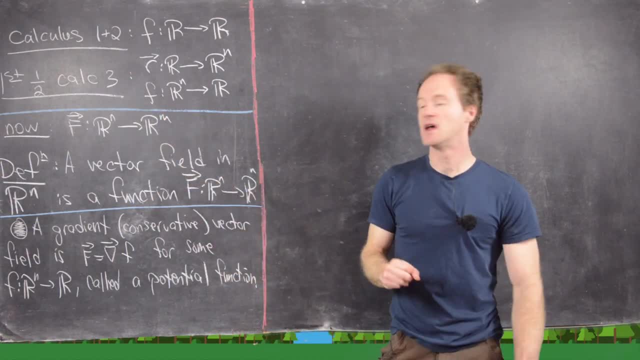 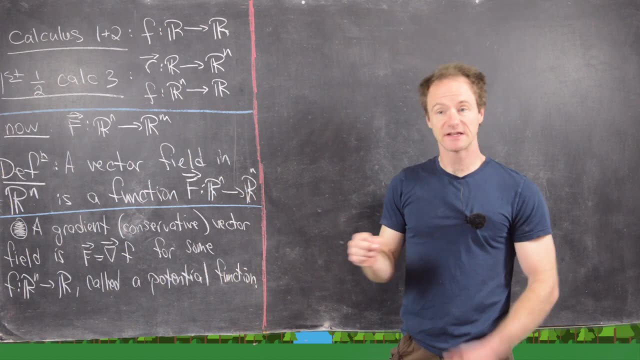 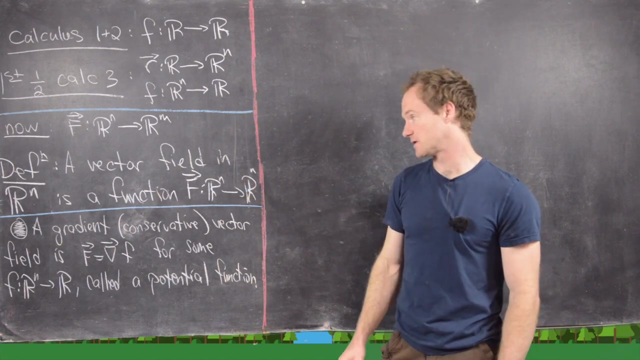 So you deal with this kind of thing in linear algebra. it'll be like an m by n matrix, but this is not something that we'll deal with This course, although you can generalize it quite easily to this. what we will deal with is something that's called a vector field. 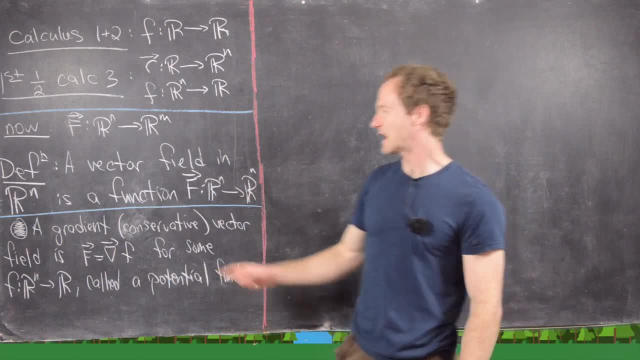 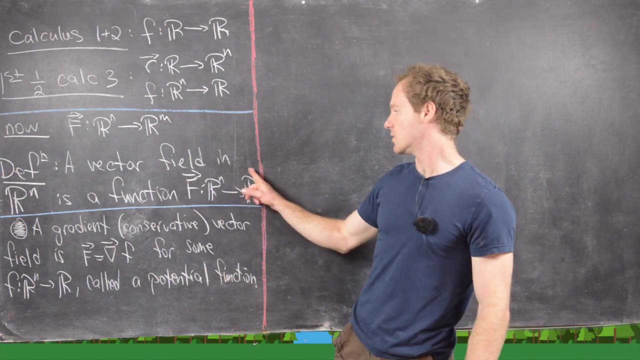 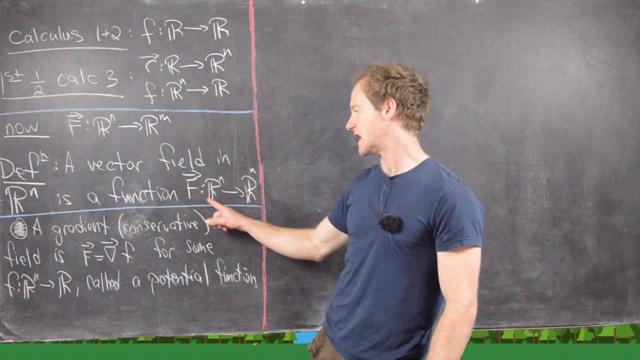 And the definition is pretty simple. So a vector field in Rn. it's a function from Rn to Rn, So we're going to keep the domain and the codomain having the same number of entries. So generally we think about the domain as having n variables. 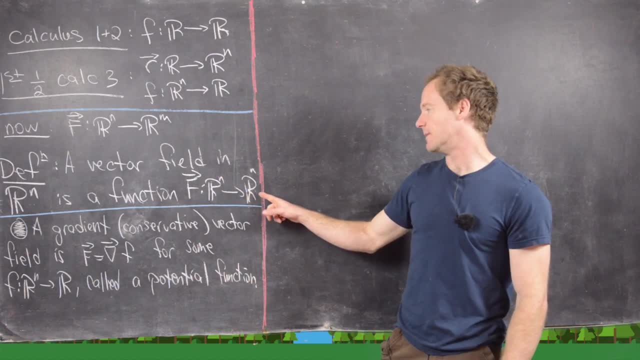 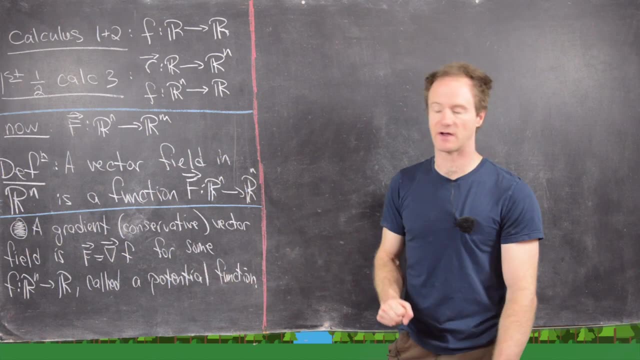 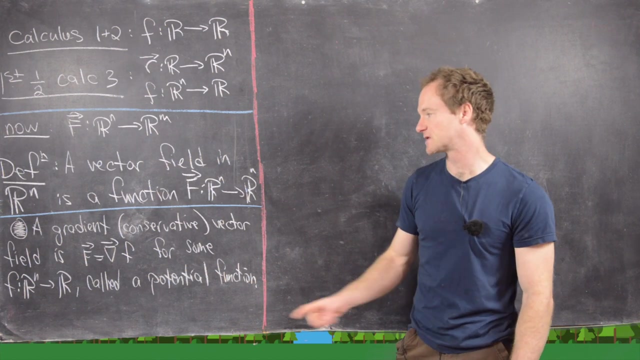 and then the output will be a vector that is n in length. Okay, great. And then one special type of vector field is called a gradient vector field. So sometimes this is called a conservative vector field, because it represents some important properties in physics. 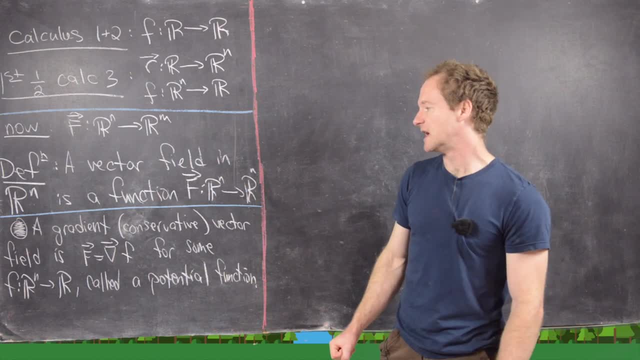 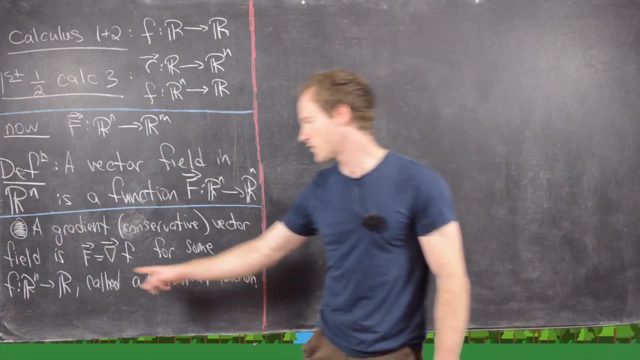 So a gradient or conservative vector field is a vector field that can be defined by taking the gradient of an invariable function. So in other words, F, capital, F, I should say, is the gradient. It's the gradient of little f. 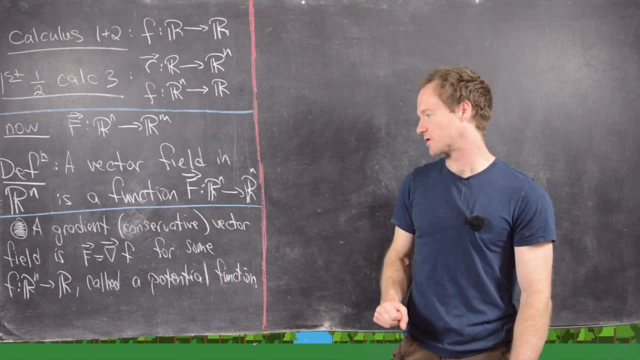 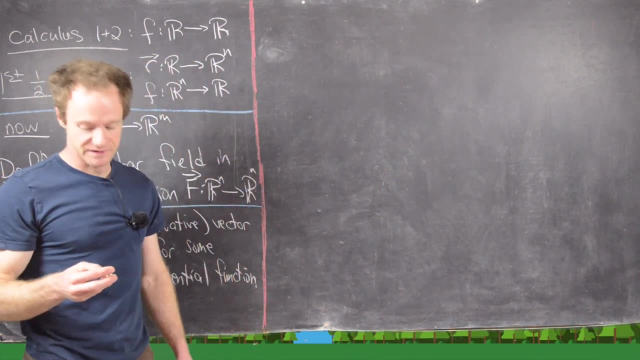 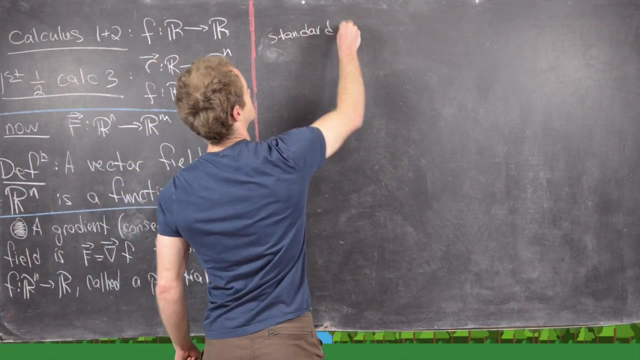 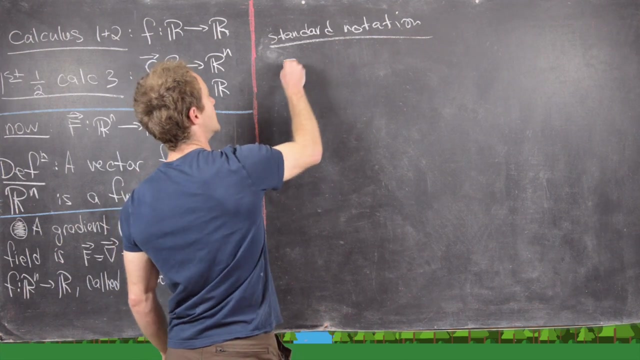 And little f is a multivariable scalar valued function, And so that function f is called the potential function. Okay, so before we do some examples, I want to give you some standard notation for vector fields, And standard notation for vector fields in R2 is as follows: 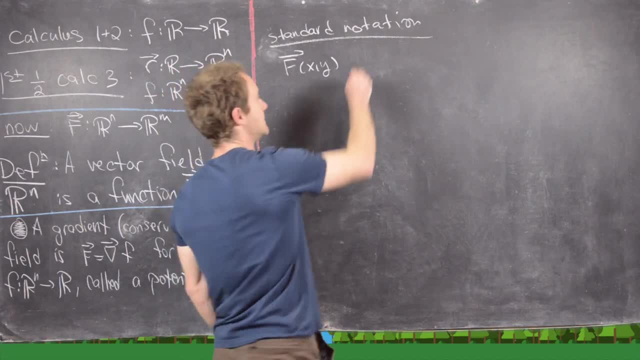 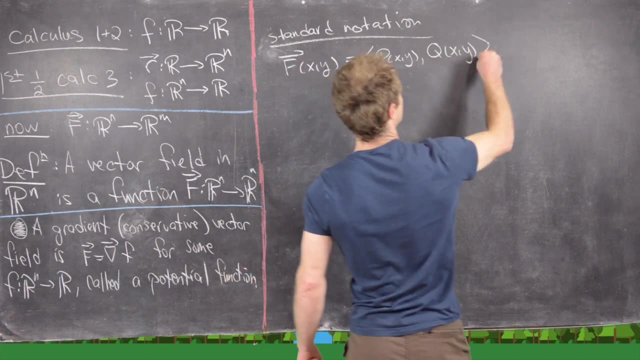 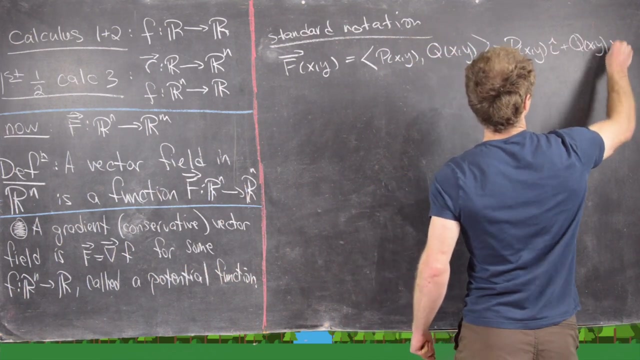 So generally we'll write f of x- y, And so this will be the vector field built by p of x y, q of x? y, Or maybe p of x? y in the i direction plus q of x? y in the j direction. 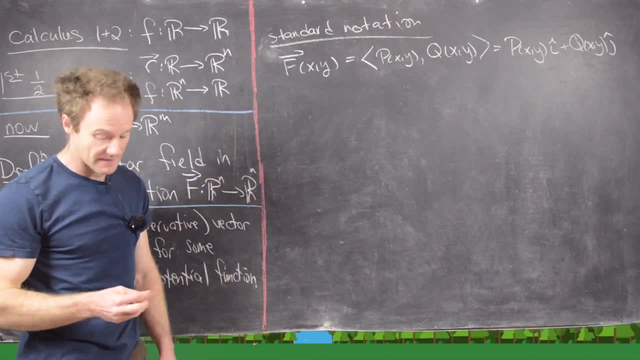 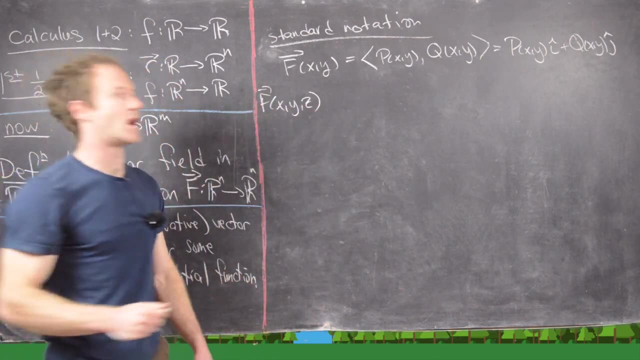 It's pretty common to see them in both ways. And then if you have a vector field in R3, so that means you need three inputs- x, y and z- And that means you'll also have three outputs And we'll call those p of x. 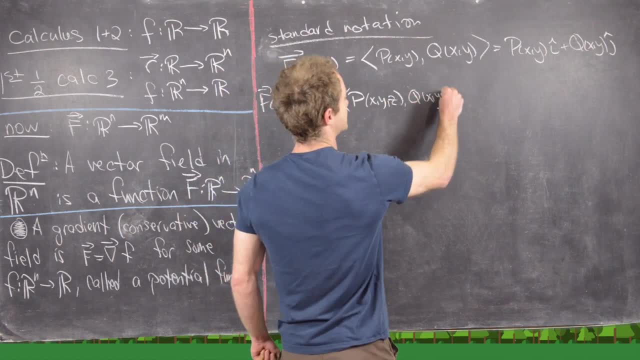 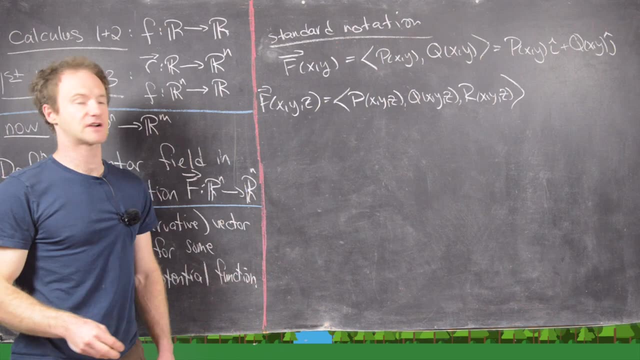 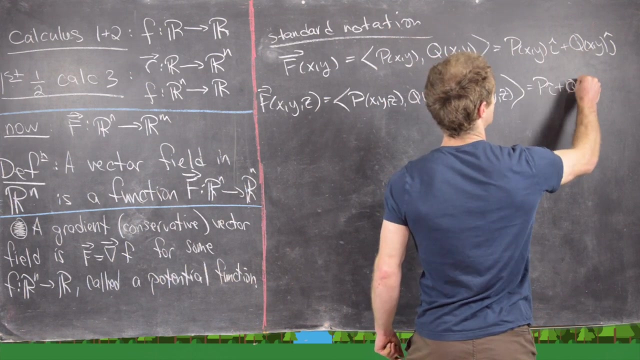 y z, q of x y z and r of x y z. So that's the standard notation for a vector field in R3.. And usually we'll write p in the i direction, q in the j direction. 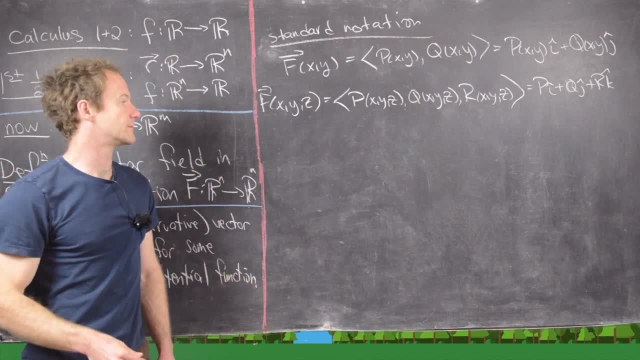 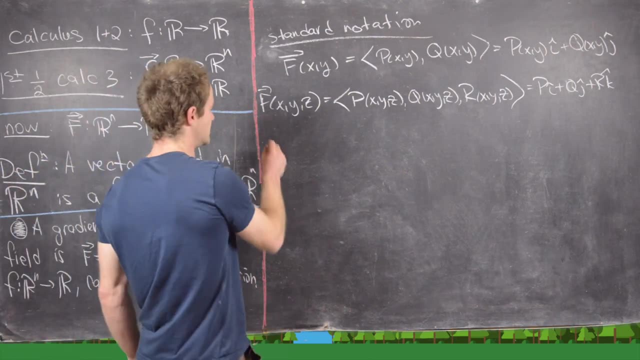 and r in the k direction, Something like that. Okay, so now I want to look at some graphical representations of vector fields, And we'll start with a pretty simple one. So the first one that we'll look at is f of x, y. 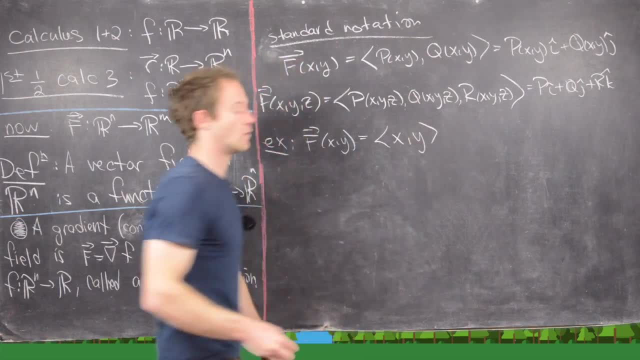 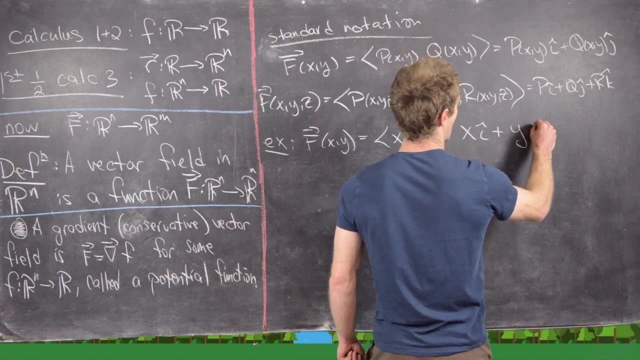 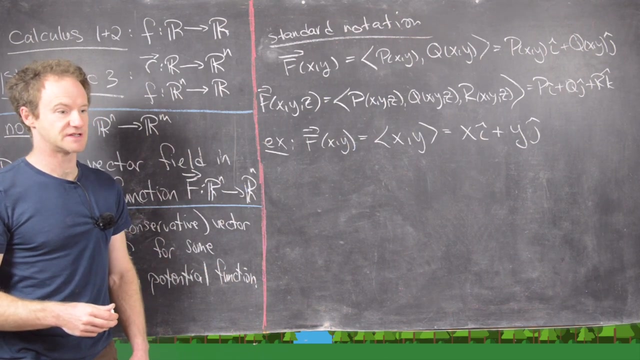 equals the vector field x, y. So notice that this thing can also be written as x in the i direction plus y in the j direction. Okay, So you might think: well, how can we look at a graphical representation of this? Because essentially we have four dimensions. 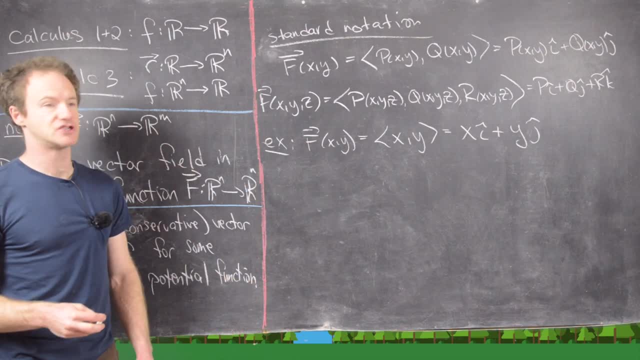 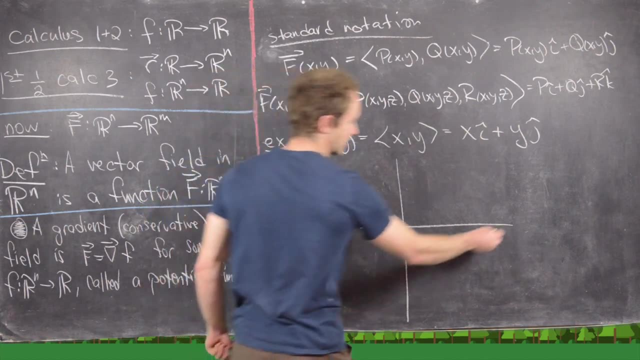 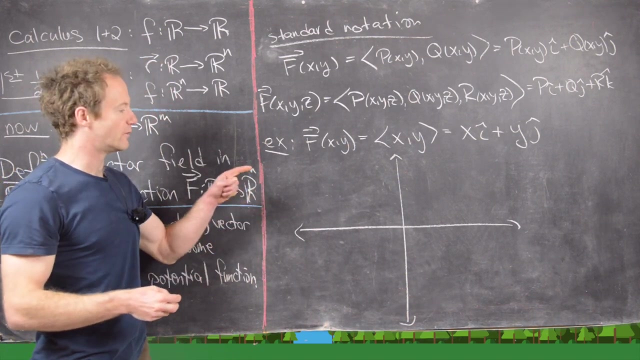 We have two domain dimensions And, uh, two range dimensions. But we can do it in the following way: So we'll draw the x? y plane like this, And then, at selected points in the x? y plane, we will draw a vector. 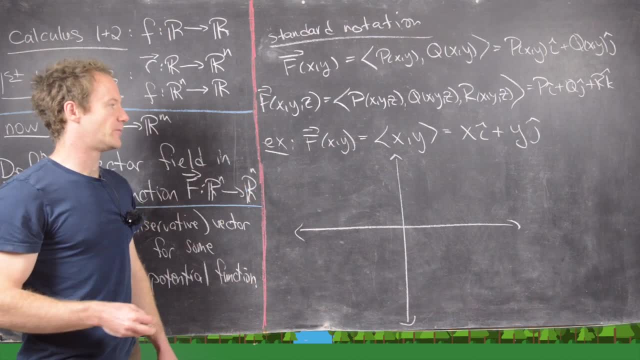 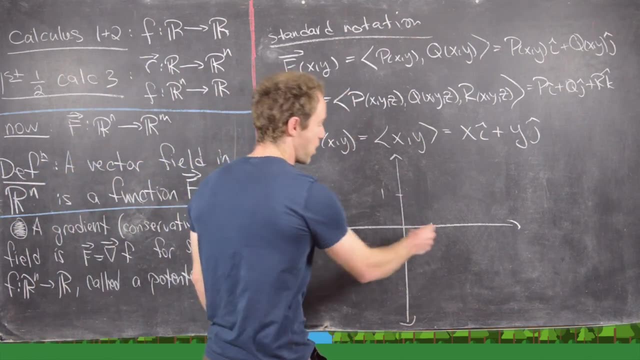 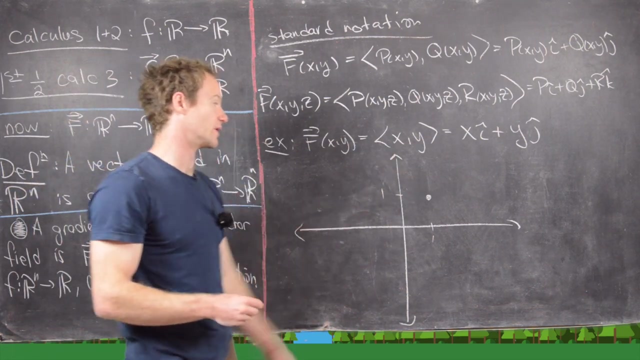 which is given by the output of this vector field at that point. So, for example, if we go here to 1, 1, we'll go up here. now we want to plug 1, 1 into this vector field. Notice that's also going to give us 1, 1.. 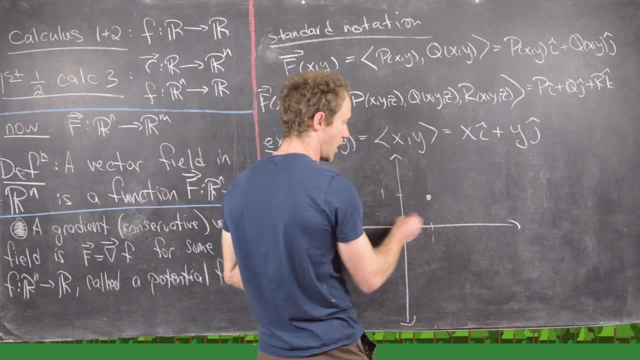 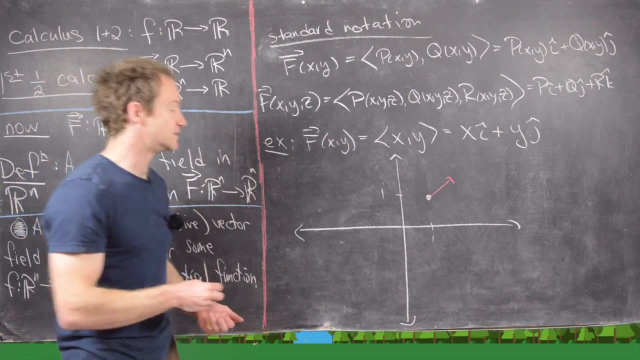 And then what we'll do is we'll draw the vector 1, 1 at this point, So we'll get something like that, And then what we'll do is do that at every point. So, uh, let's go ahead and draw down here. 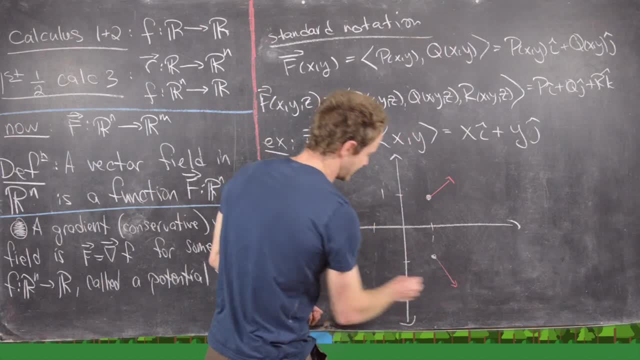 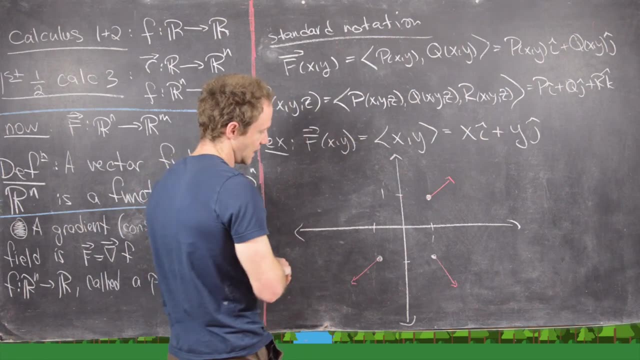 which is like 1, negative 1.. So that'll give us that vector, And then negative 1, 1.. So that'll give us that vector. Um, and then finally, uh, negative 1, 1.. 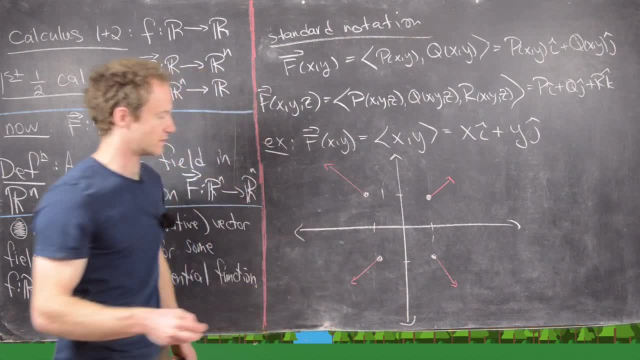 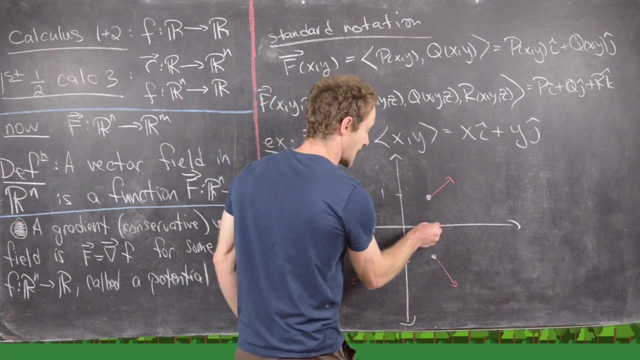 So that will give us, uh, this vector pointing up this way. Okay, good, Now let's look at some other ones. So notice, along the x-axis. we'll just have a vector pointing straight along the x-axis to the right or to the left. 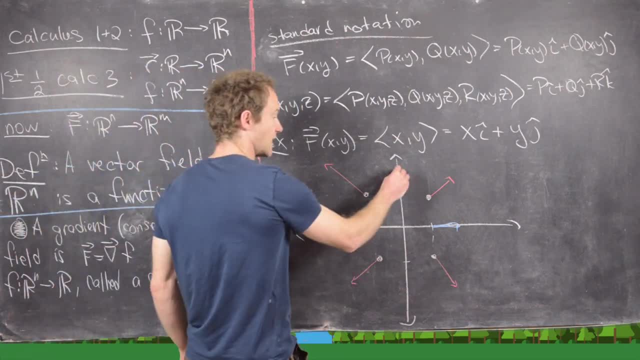 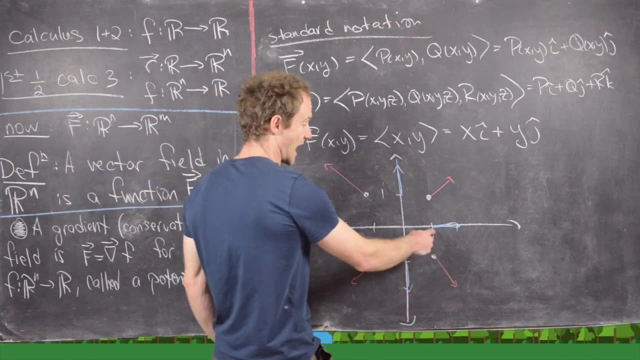 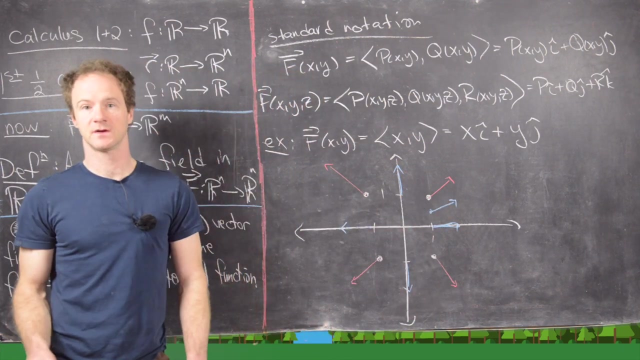 depending on if we're in positive or negative values of x, Here we'll have vectors pointing up or down. Okay, great. And then notice, maybe here at 1, 1 half, we're gonna be pointing in that direction. Good. 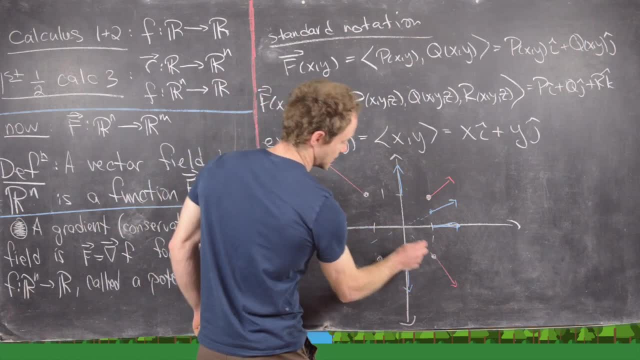 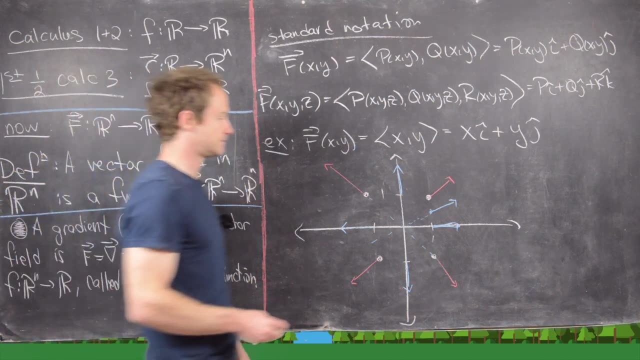 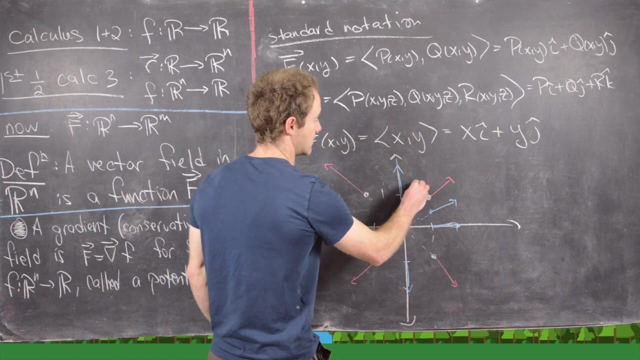 And notice that all of these vectors lie on uh lines radially emanating from the origin. So we'd have another one right here pointing up that way. Okay, great, So you can think of this as like some sort of explosion going out. 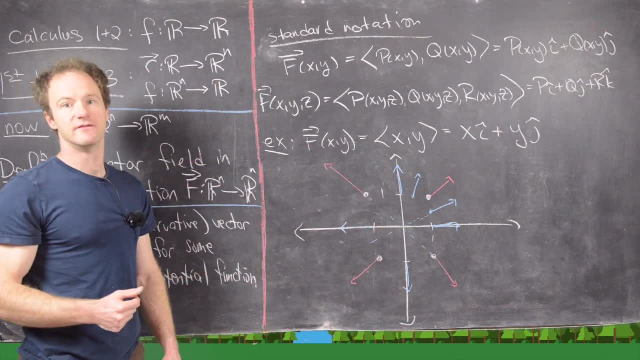 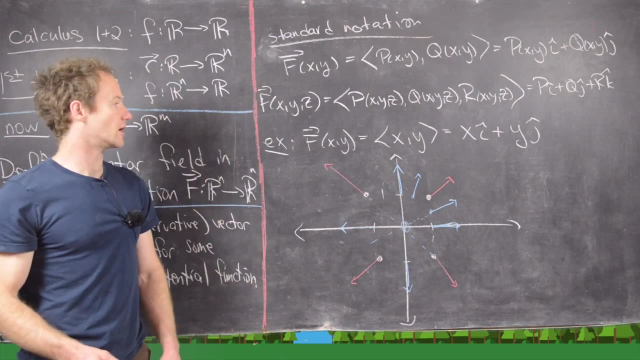 We have a radial um picture of vectors emanating from the origin And notice down, here is the only time you get, uh, zero vector for um the vector field. Okay, great. So I'll clean up the board and then we'll look at a couple more graphical. 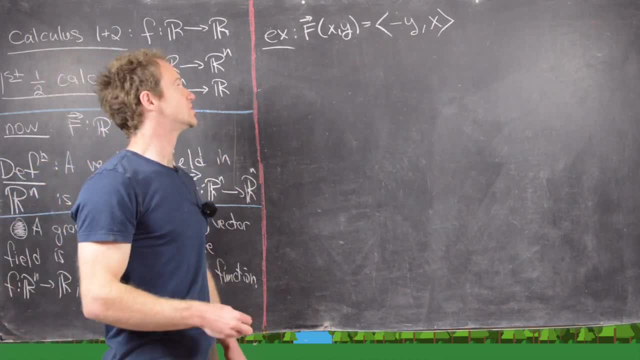 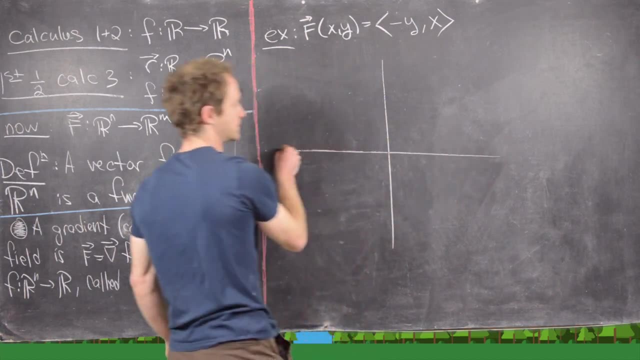 examples. So the next one I wanna look at is this one right here, which is f of xy equals negative yx. So, uh, let's get a picture of this going, Okay. So I'm gonna go ahead and put a couple of points here. 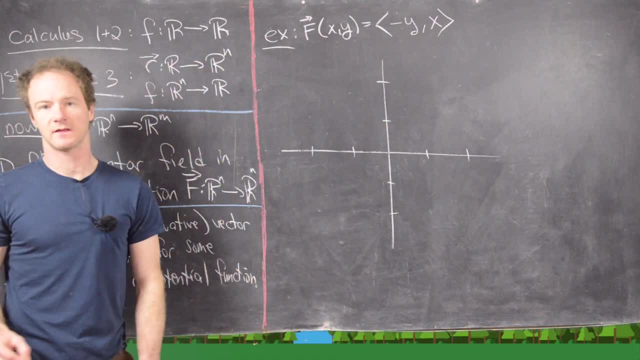 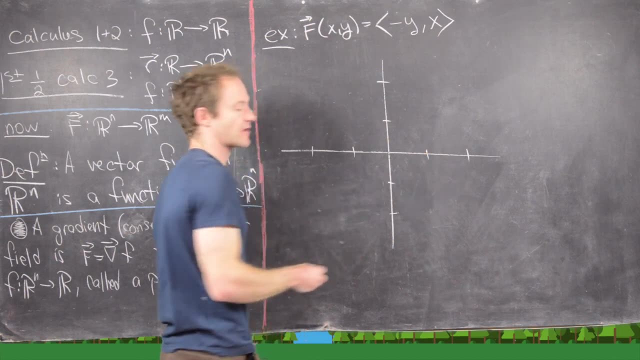 Let's put points along the x-axis like that and the y-axis Okay. So notice here at the point 1, 0, if we plug 1 in for x and 0 in for y, we will get the vector. 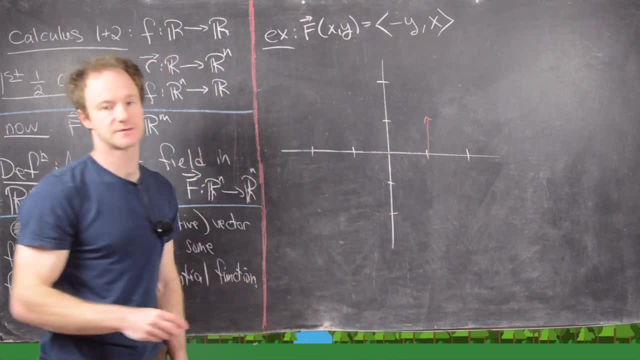 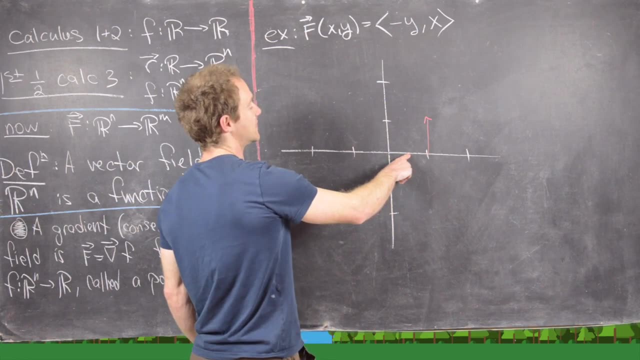 0, 1.. So that thing is pointing up here like this: Okay, good Now, uh, let's notice back here at 1, x 0, 1.. If we plug 1, x 0 in 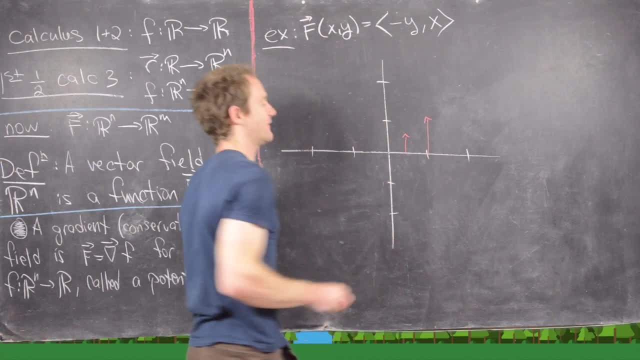 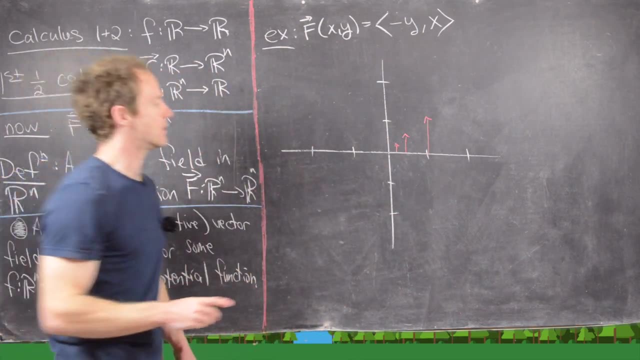 we get the vector 0,, 1, x, So we'll get about half of that. And then if we plug in a quarter, we'll get a quarter of that, and so on and so forth. Okay, now if we plug 2 into this, 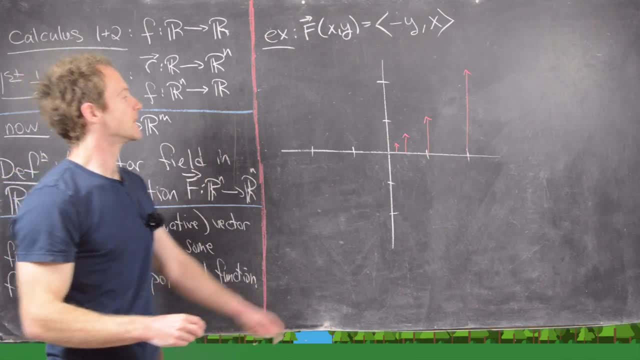 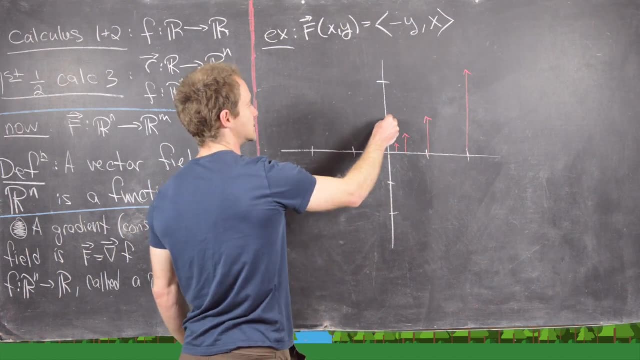 we'll get twice that vector. Okay, great. Now notice, if we plug in the point 0, 1,, we will get the vector negative 1, 0.. So that's gonna be the vector pointing this way. Okay, good. Then if we plug in the point 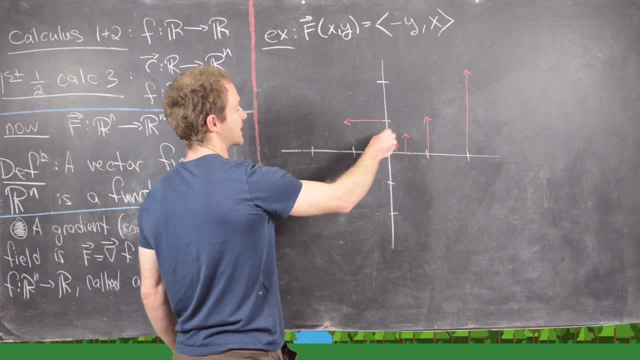 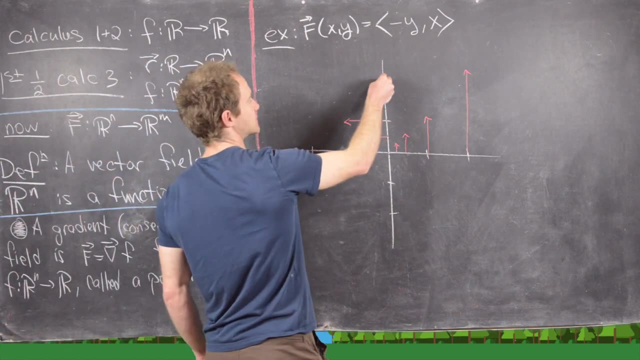 half, sorry, 0, half. we'll get this vector pointing back in this direction. So we'll get negative, half, 0, that vector Good. And then notice, right here we'll get a vector pointing back, uh, 2 units. 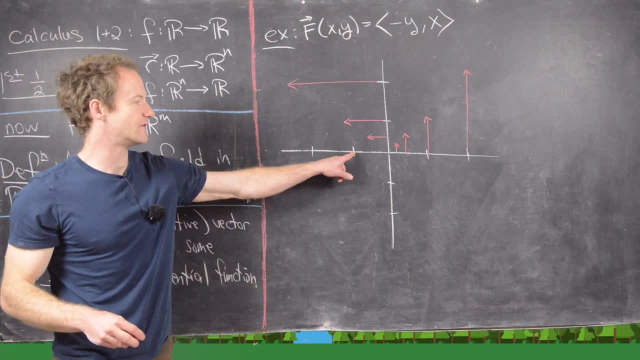 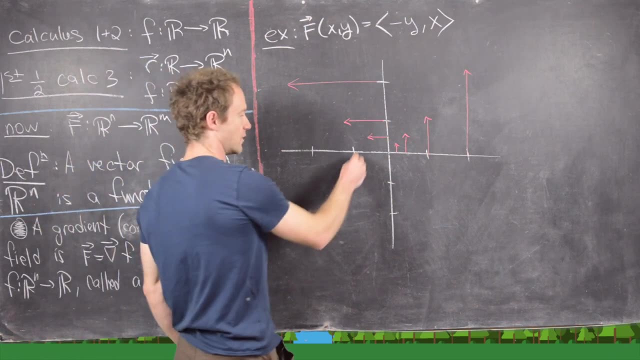 Okay, Now let's look right here. So this is the point: negative 1, 0.. So if we plug negative 1, 0 into this, we will get uh 0, negative 1.. So that's gonna point. 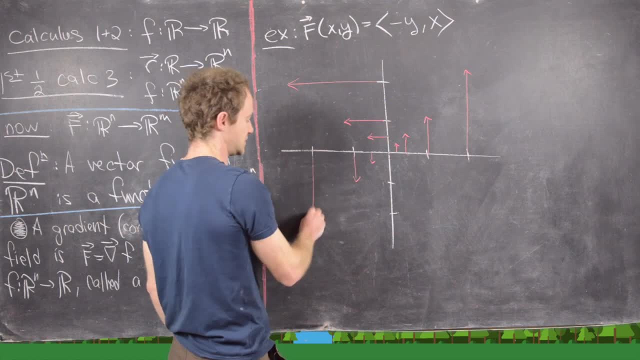 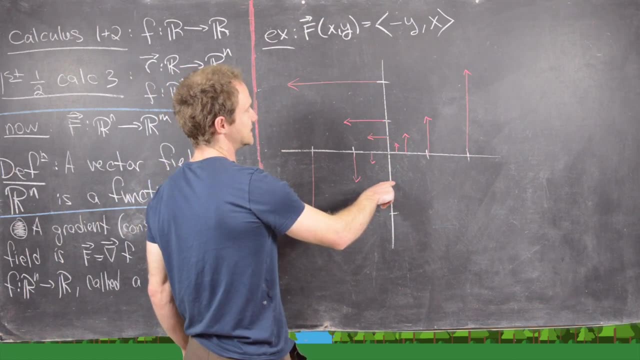 down, And then if we do half, it's gonna be like that, And then if we do 2, it's gonna be a little bit longer. Okay, great, And then let's try this one. So if we plug 0, negative 1 in. 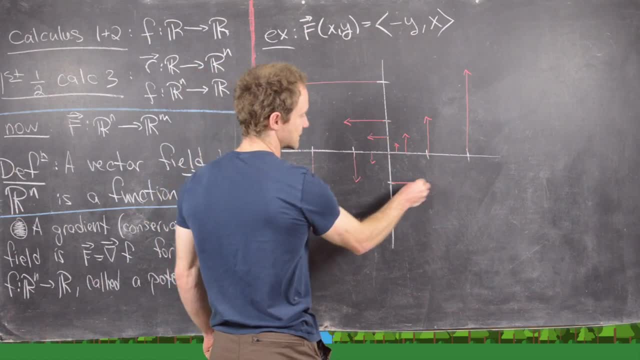 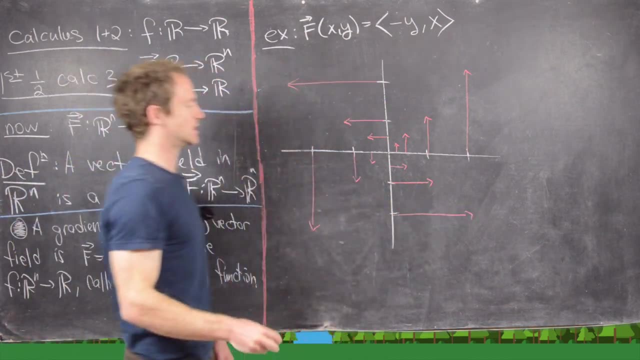 notice, we're gonna get the vector 1, 0.. So that's gonna point in that direction. If we do a half, we'll get kind of the same thing, And if we do 2, we'll get the same thing, but longer. Okay, so 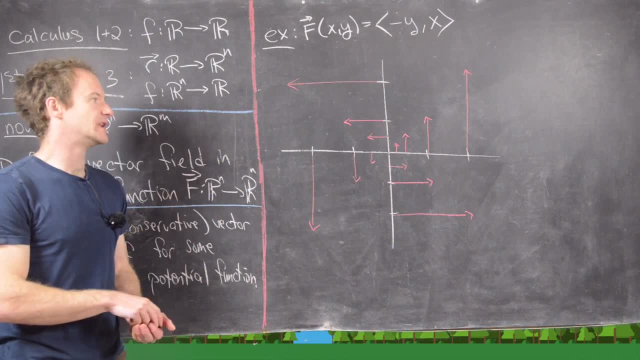 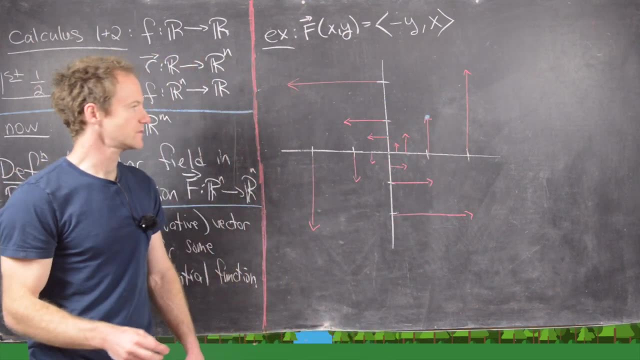 that's what our vector field looks like along the coordinate axes. Now let's look at some other points. So let's maybe go up here and look at this point 1, 1.. So if we look at this point 1, 1,, 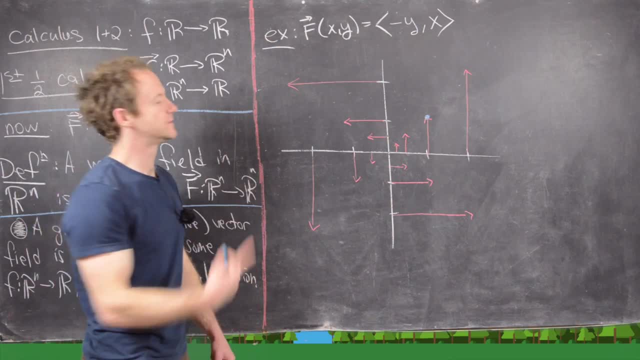 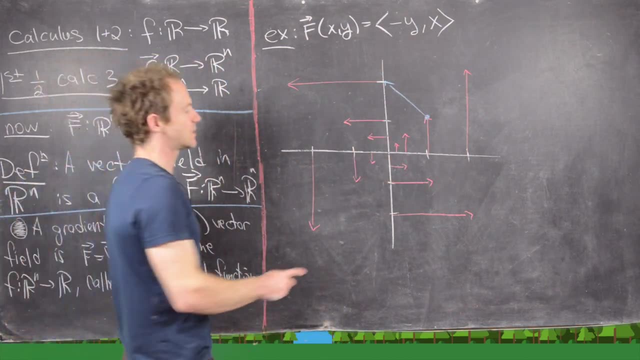 we will get the vector uh, negative 1, 1.. So notice the vector negative 1, 1 is pointing back in this direction. Okay, good, Now let's go ahead and look at the point um. let's see what this is. 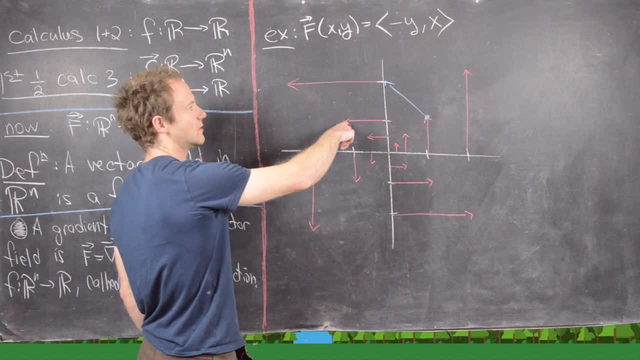 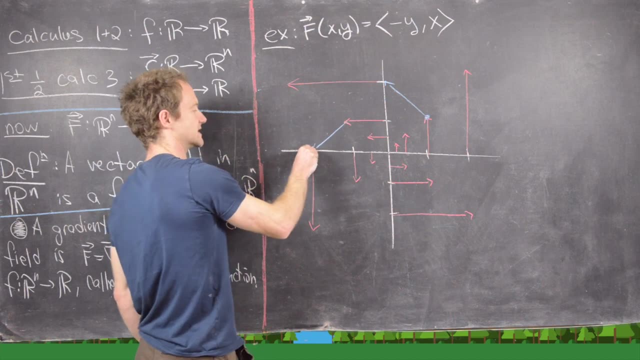 Negative 1, 1.. So if we look at the point negative 1, 1, that's going to turn into the vector negative 1, 1.. So that's going to take us down like that. Okay, good, And then. 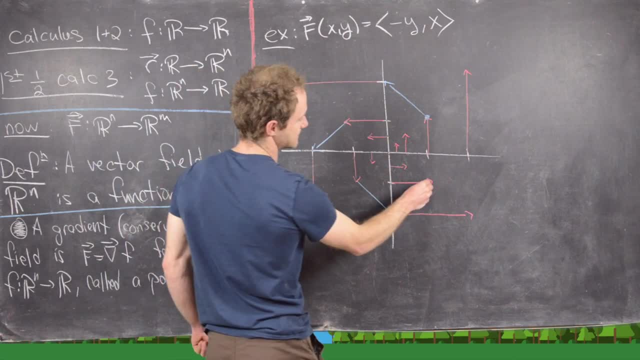 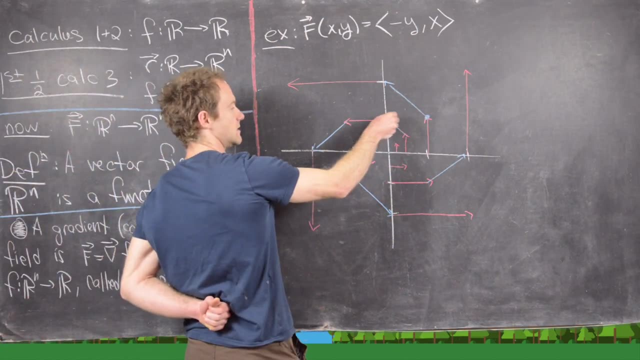 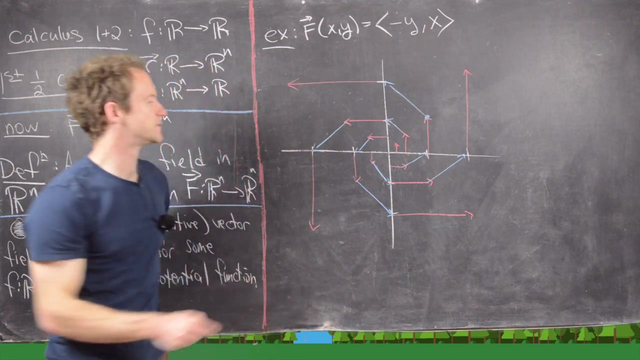 similarly, this guy is going to take us down like this and this guy is going to take us like that, Okay, great, And now, uh, we can also kind of fill in those spots, Good, So, as you can see, we kind of get. 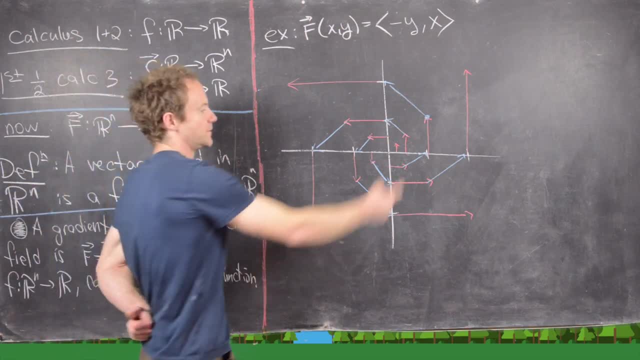 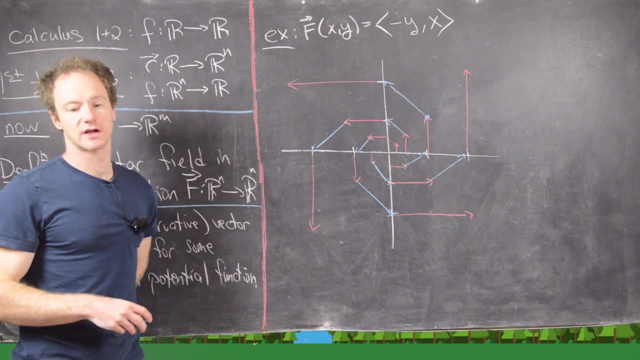 a spiral in this case. So, um, the vector field is pointing around in a circle. Okay, great, So I'll clean up the board, and then we're going to look at one more graphical example. Okay, for our last graphical example. it looks pretty. 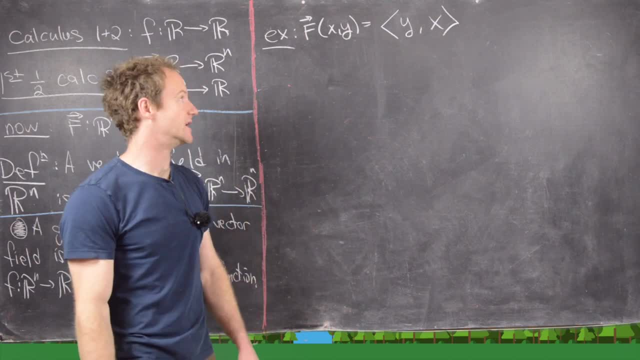 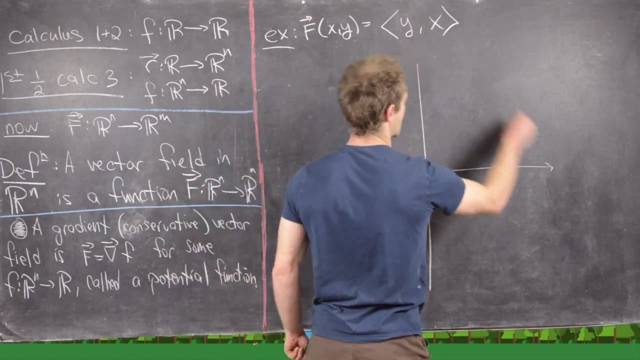 similar to the last one, but I've erased the minus sign. So I have y x. So let's go ahead and draw our picture here. So let's see, we have our x y plane. I'm going to put 1 and 2 on both. 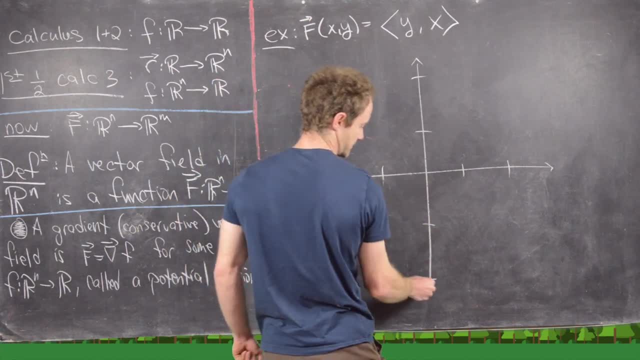 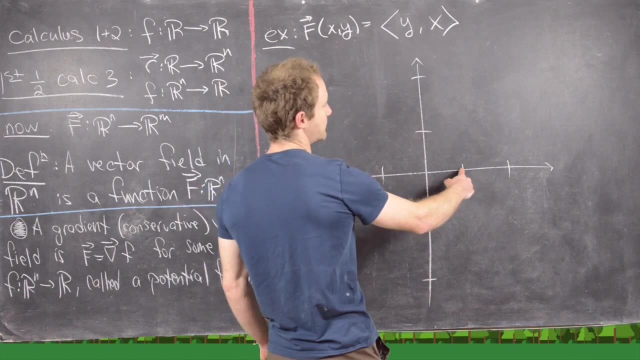 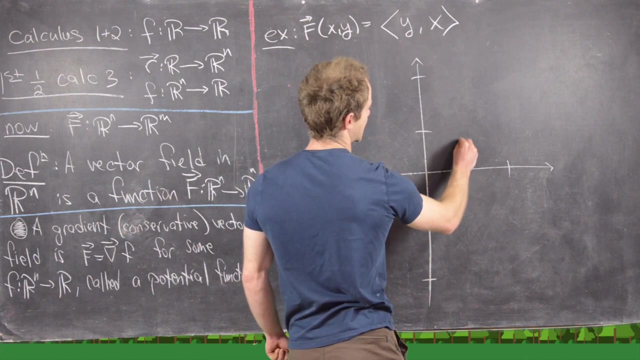 of the axes just for us to work with. And now let's see what we get along: the coordinate axes. So notice over here. this is the point. So that's going to turn into the vector. So, in other words, that's going to. 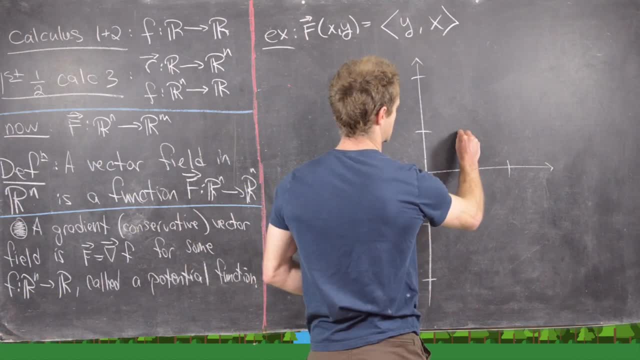 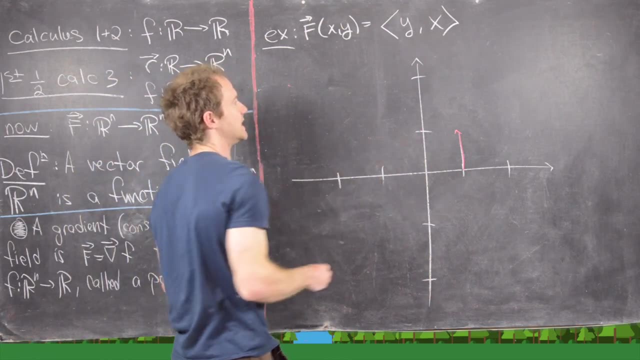 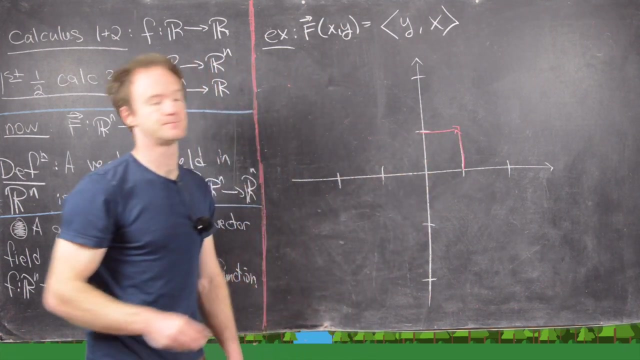 be pointing up like that: Okay, good Now, uh, let's go over here and notice this is the point and that's going to turn into the vector. so that's going to be pointing that way. Okay, and if we go down here, 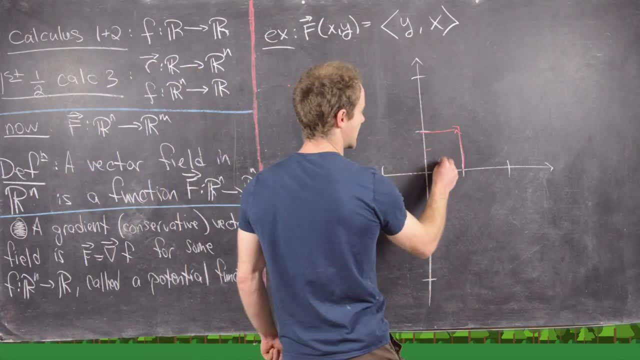 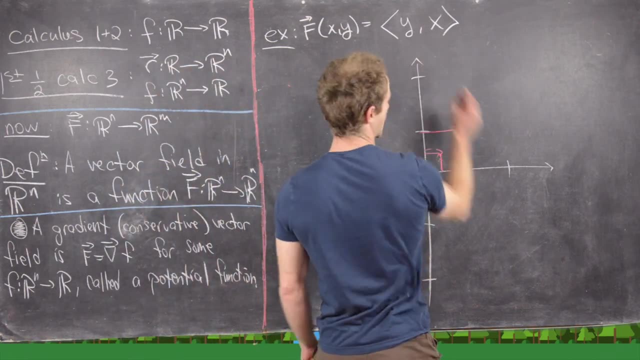 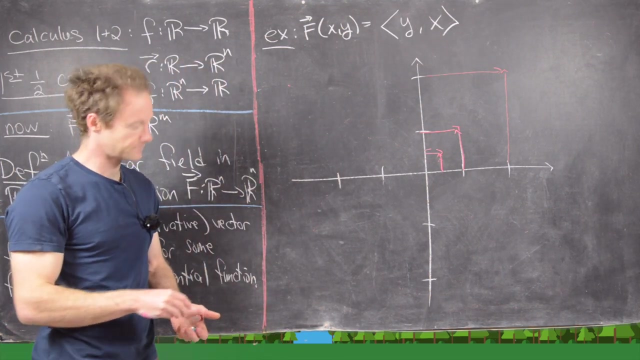 to a half, we'll get the same thing, but these are just units, So those point towards each other- Great. And then, if we do two, we'll get the same thing, but those are pointing towards each other like that, So we get something like this: 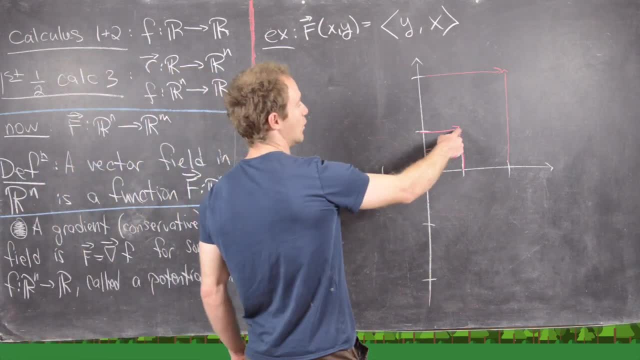 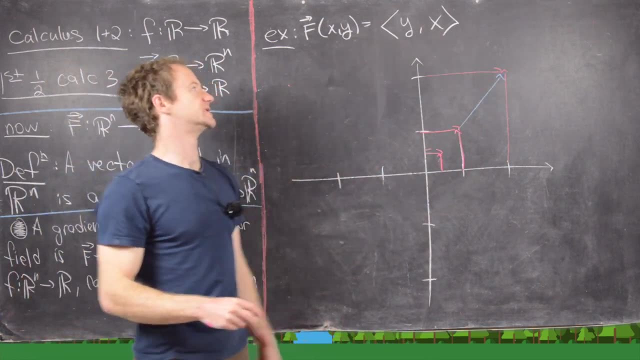 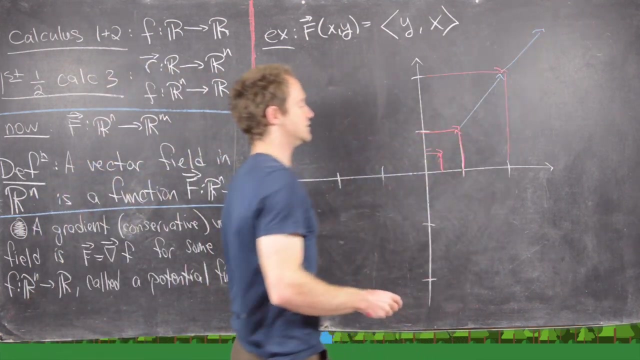 Um, okay, great, Now let's see what's happening at. So notice is going to be pointing in that direction, Because all we do is switch the order of and, but switching the order of just gives us, And, similarly, if we do, 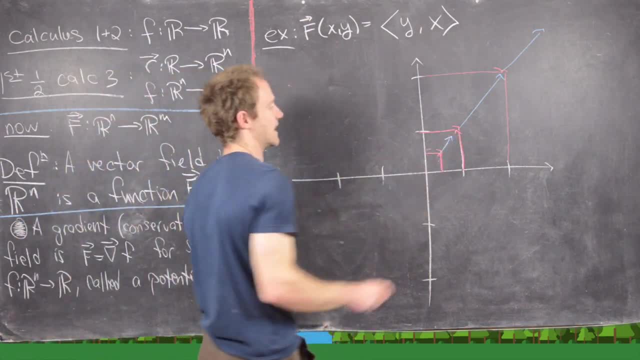 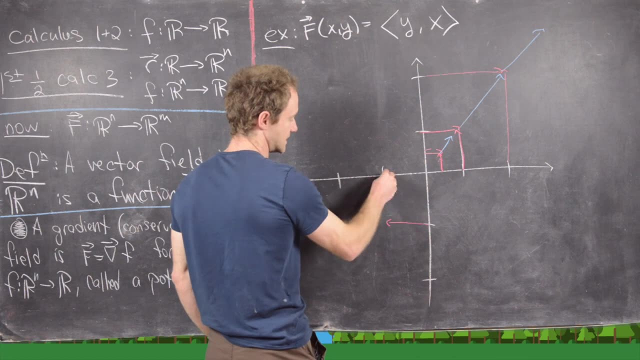 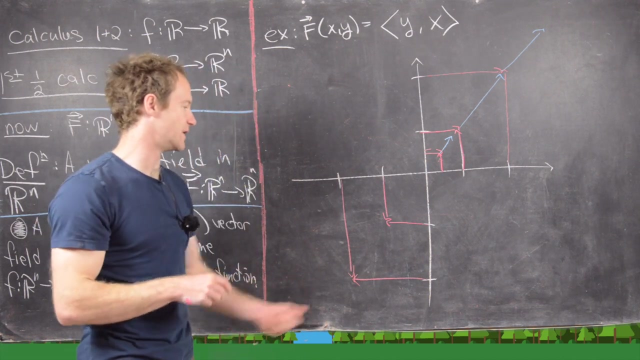 it's going to go like that. If we do, it's going to go like that. Okay, great. Now, um, by some symmetry, we have the same thing going on down here, So I'll let you guys fill that in, but notice. 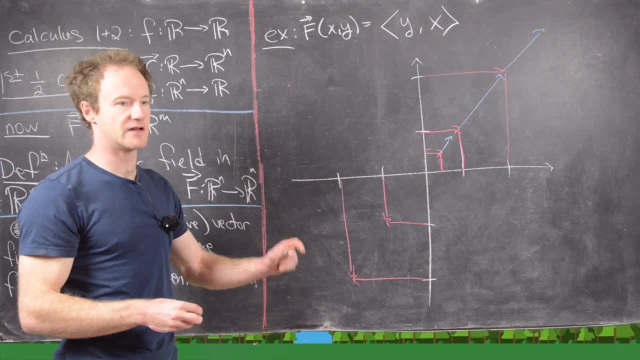 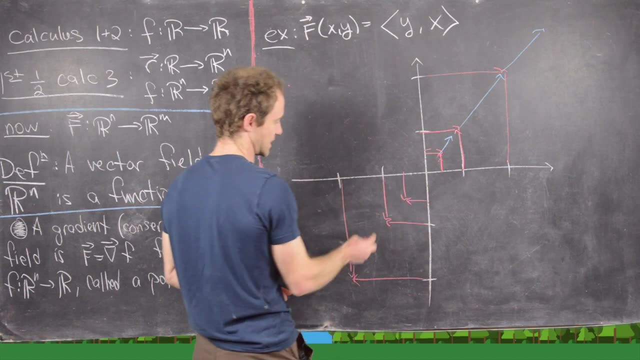 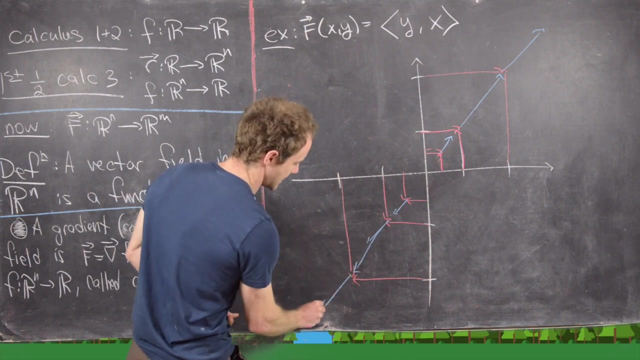 over here in the third quadrant, x and y are both negative. So, um, you get this same kind of picture, Uh, it's just pointing in the opposite direction. So we get something like that and then, along this line, we'll be pointing away like 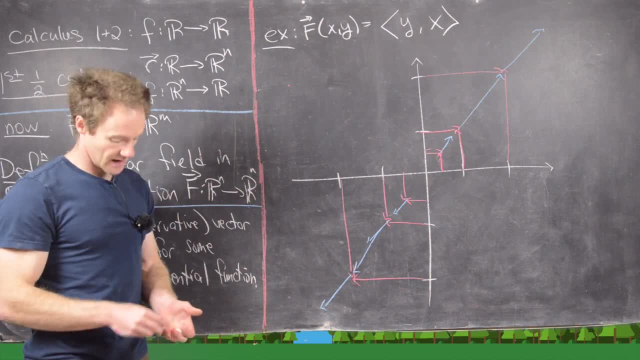 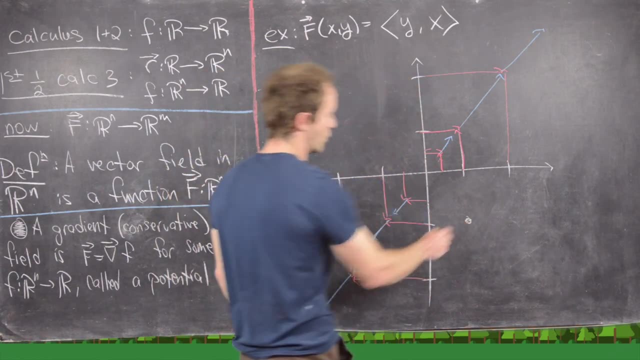 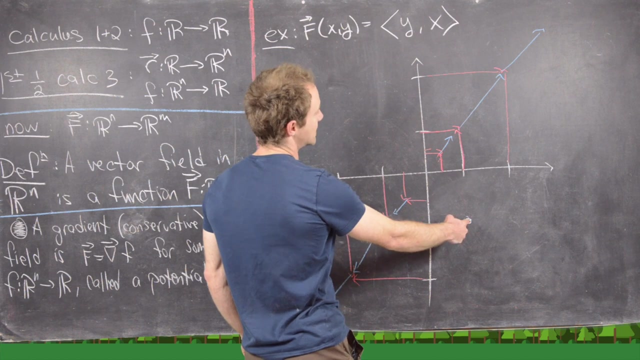 this. Okay, great Now. uh, the next thing to notice is maybe what's happening over here, like at the point, So at the point, that's going to switch to the point and so that's going to be pushing back towards the origin. So we 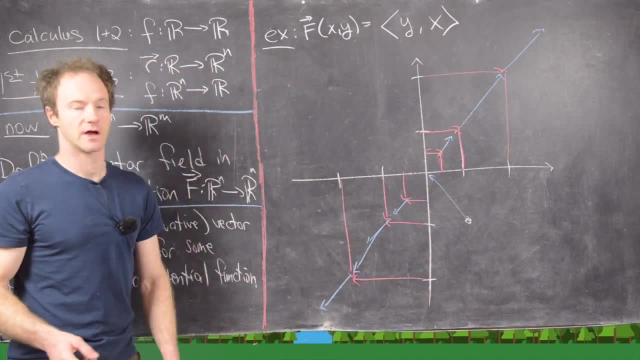 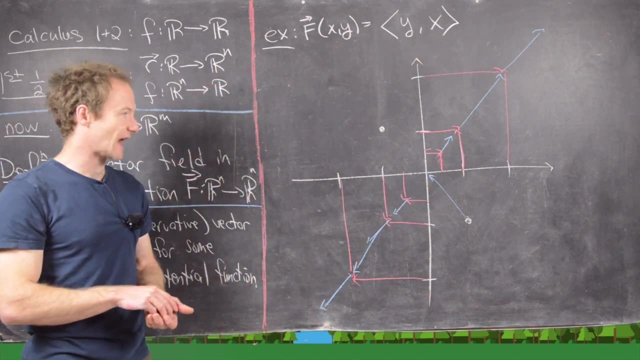 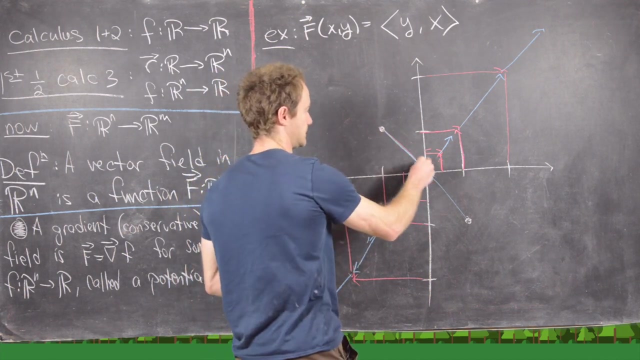 can draw that like this: Okay, great. And then similarly here at the point that's going to turn into the vector and that's going to be pointing back at the origin as well- Good, So we've got something like that going on, And this: 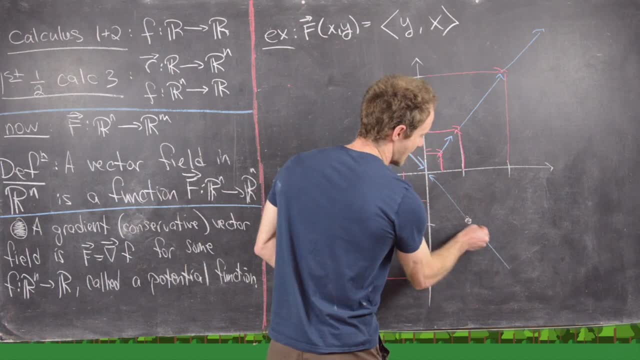 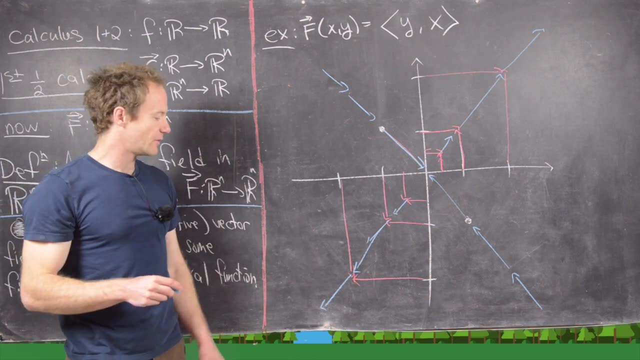 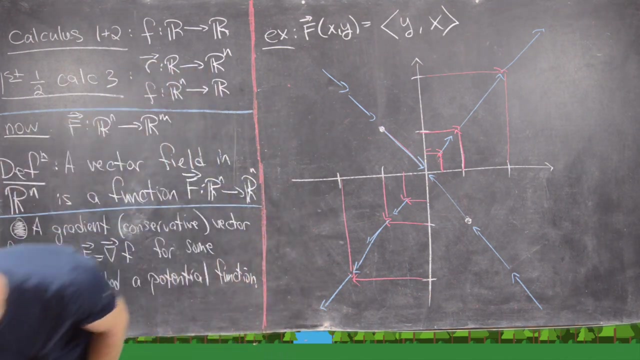 pointing back towards the origin will happen at every point along this diagonal line. Okay, so now I think we have a pretty good feel for what's going on. I'm going to draw in something called a flow line with a different color, Okay, 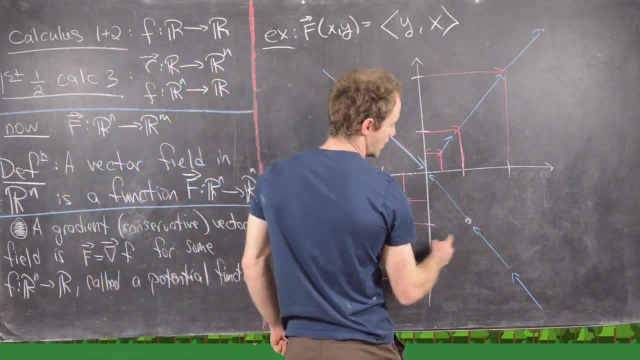 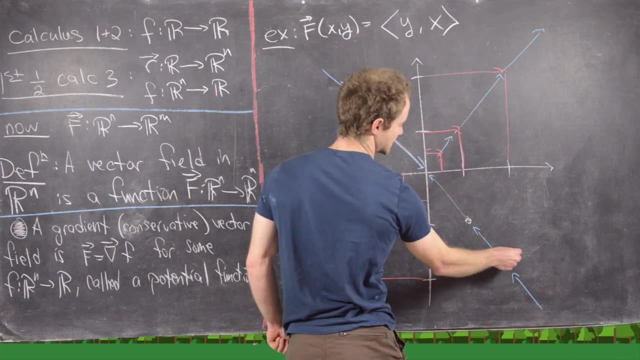 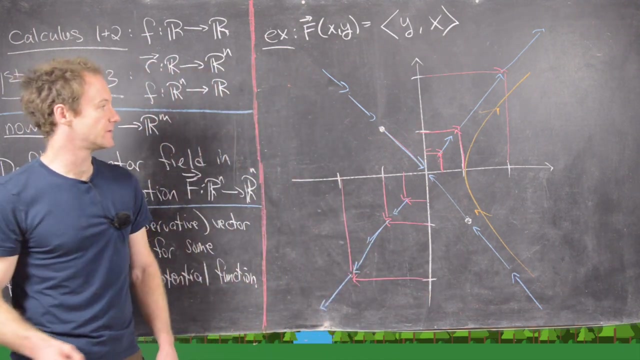 So let's notice that if you are in this region, the vector field will push you in this direction, towards this asymptote. So we have a general flow like that. Okay, good, And now, if you're up here in this bit, we'll have 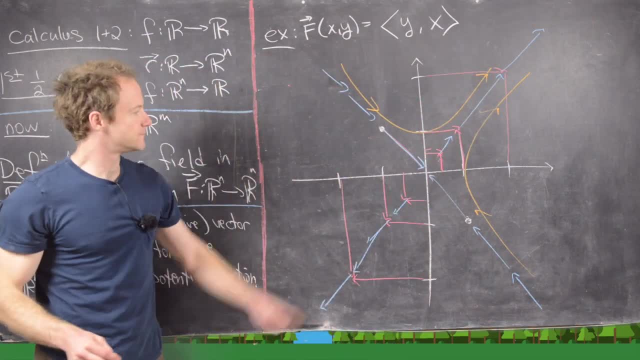 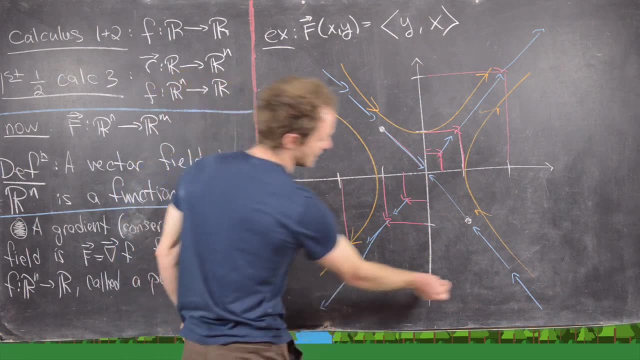 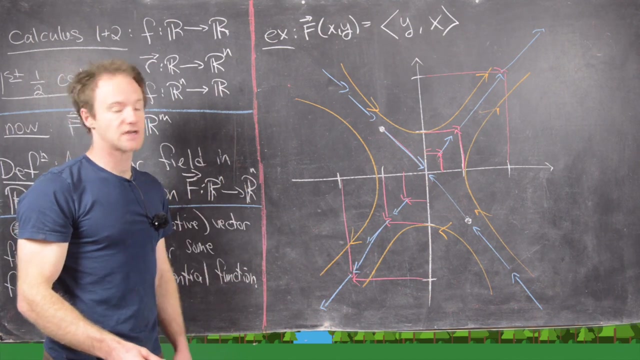 a general flow in this direction. If you're over here between these two diagonal lines, we'll have a general flow in this direction, And similarly, down here, we'll have a general flow in this direction. Okay, great, So I'll clean up the board and then we're going to do some. 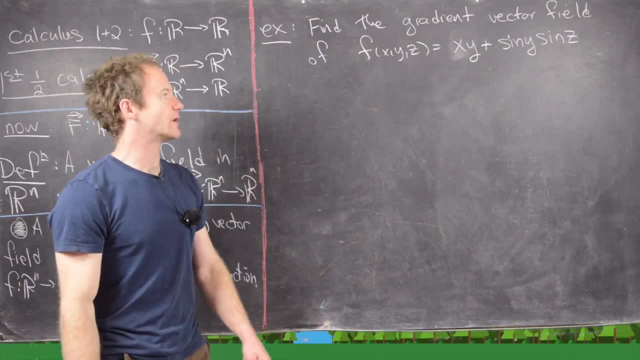 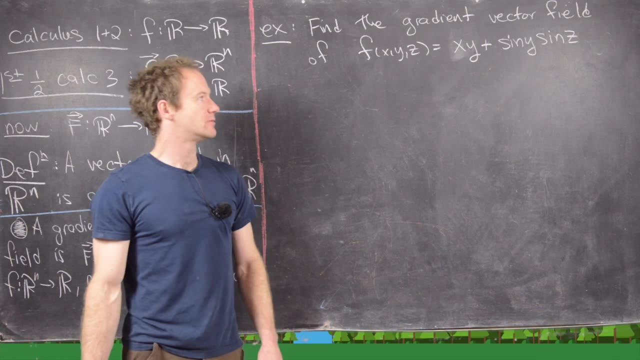 calculation type examples. For our first example, I want to find the gradient vector field with this potential function. So we have f of x, y, z equals x, y plus sine of y, sine of z. So from previously in the course we used: 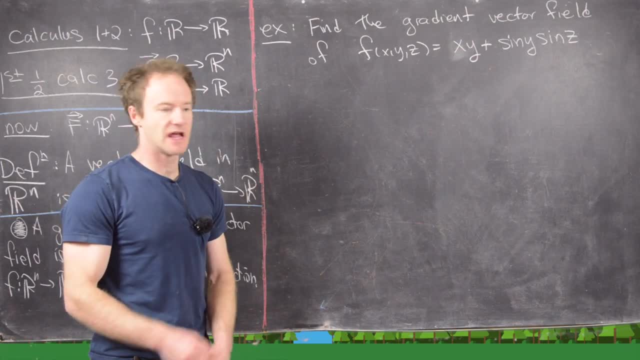 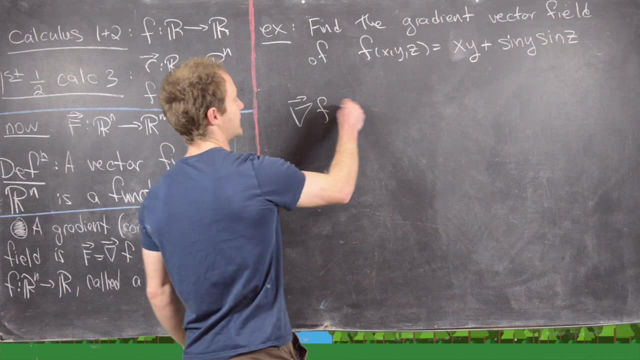 the gradient of a function in order to find directional derivatives. We've also taken lots of partial derivatives, So this shouldn't be too bad. So we need to take the gradient of f, but let's just recall that that's the partial with respect to x. 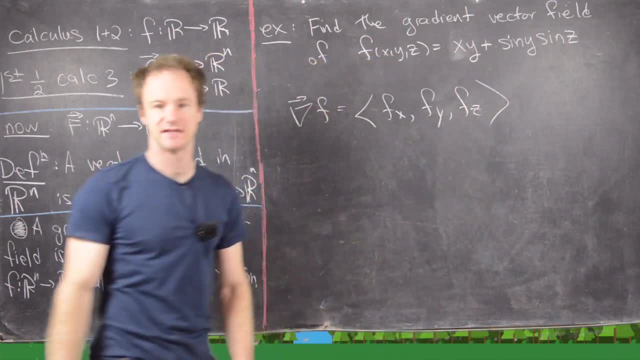 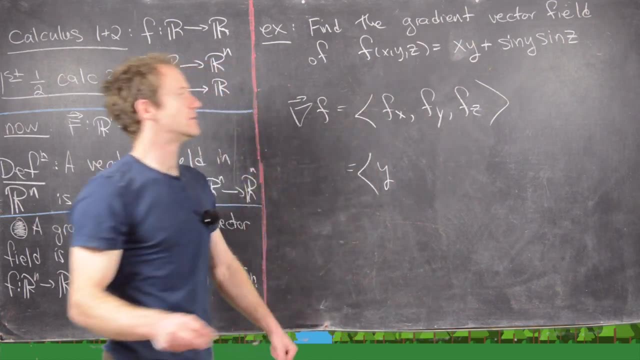 the partial with respect to y and the partial with respect to z. So let's see what we get for that. The partial of this function with respect to x is obviously y, because that second part of the sum is a constant with respect to x. The partial with respect. 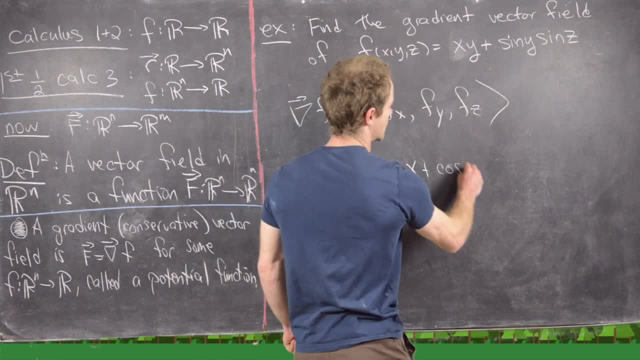 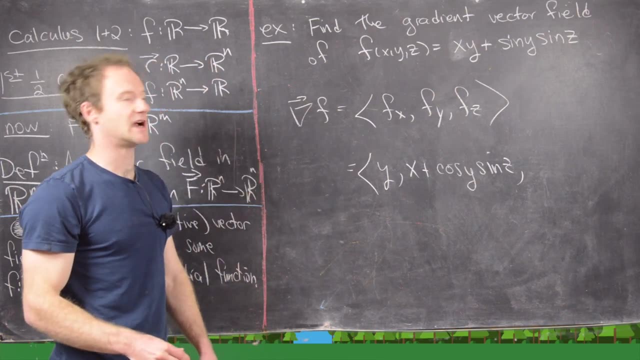 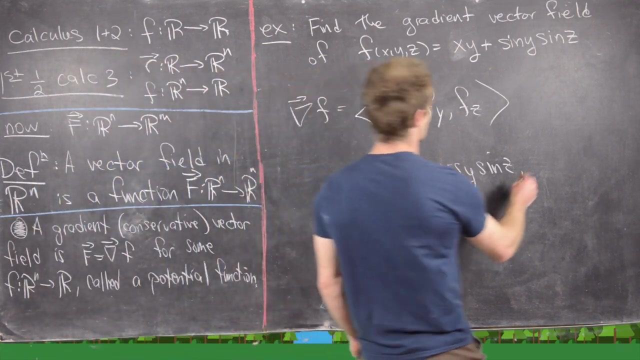 to y will give us x plus cosine of y, sine of z. So over in that second part, the sine of y is the only variable part and sine of z is a constant with respect to y. And then, finally, for this third component, we're going to get 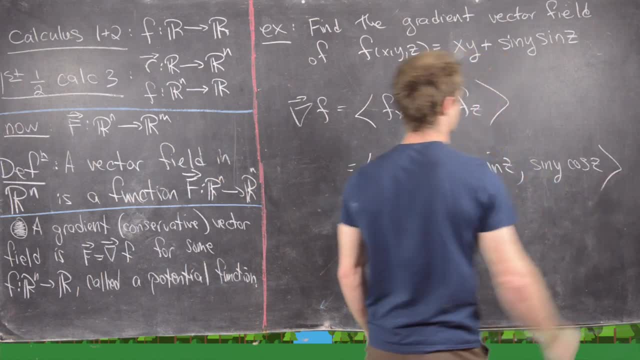 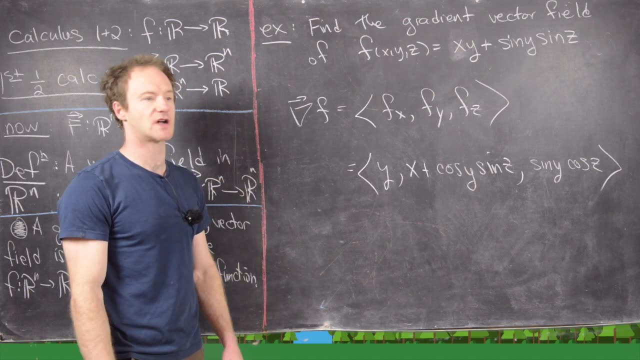 sine of y times cosine of z. Okay, so there's our gradient vector field for this potential function. Okay, I'm going to clean up the board and then we'll talk about how to find a potential function. Okay, for this next example, we're going to 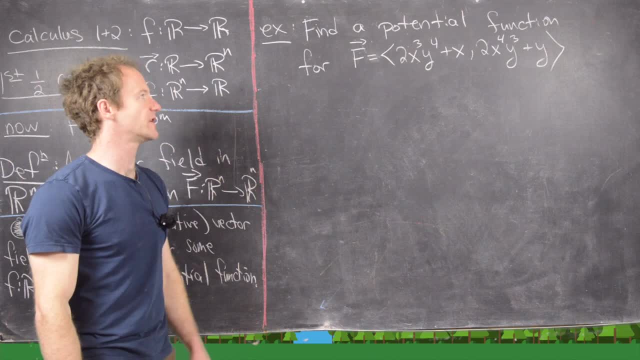 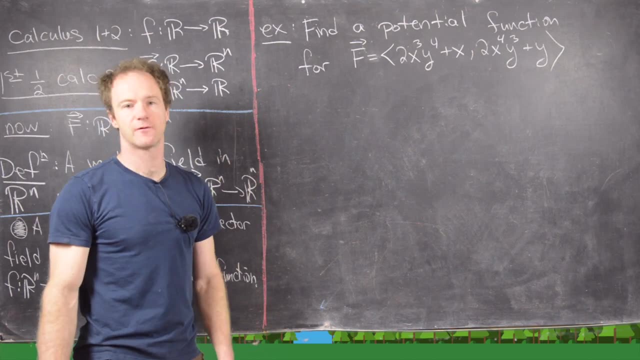 find a potential function. So the vector field that we want to work with is this: one given by two x cubed y to the fourth plus x, and then two x to the fourth, y cubed plus y. So we'll see that this is a conservative vector field. 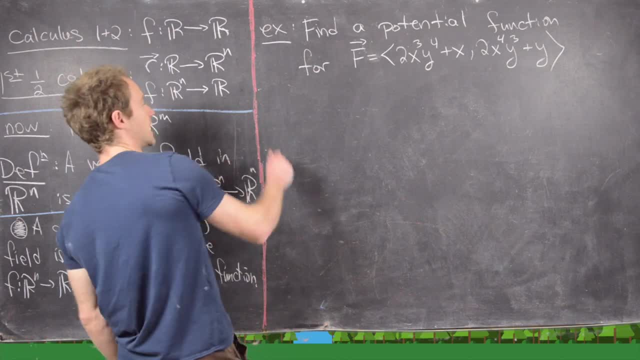 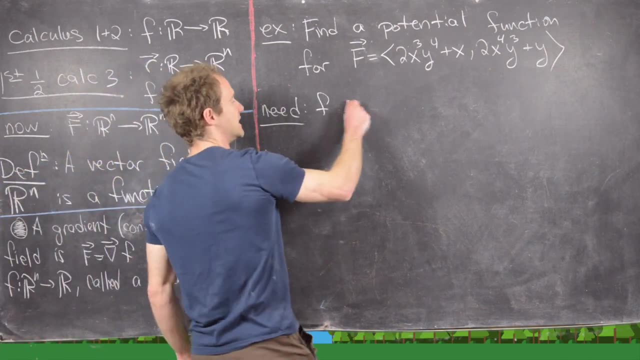 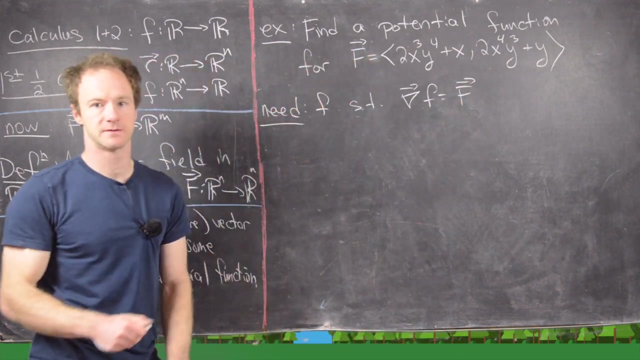 Otherwise it would be impossible to find a potential function. Okay, so what we need is we need some function f, which will be a function of x and y that satisfies this rule. So we need the gradient of f to be capital. f, that vector field. 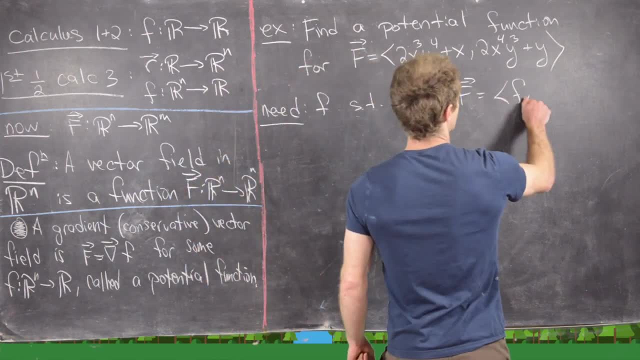 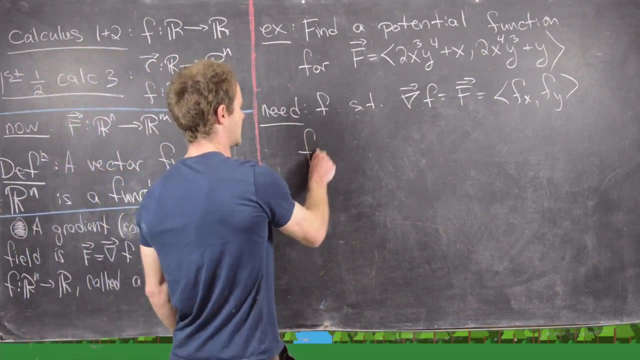 In other words, the gradient of f is given by the partial with respect to x and the partial with respect to y. So we have two equations to solve We need to solve. the partial with respect to x is got to be equal to this first component. 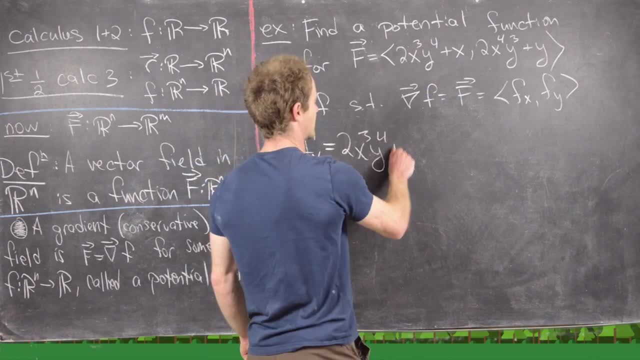 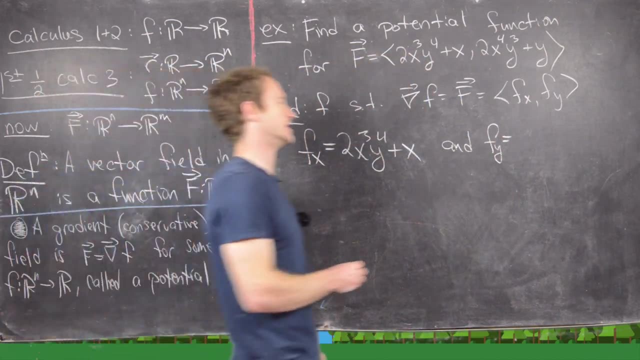 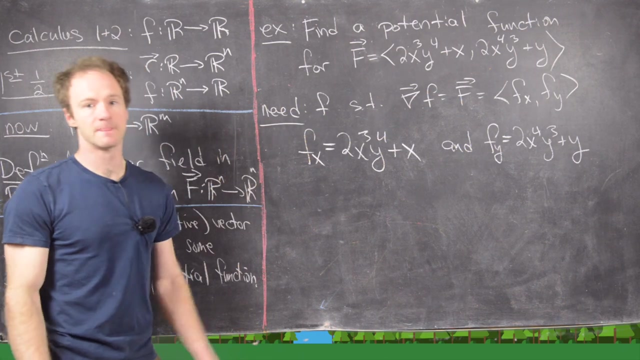 So that's going to be two x cubed y to the fourth plus x, and the partial with respect to y needs to be equal to this second component. So that's two x to the fourth, y cubed plus y. Okay, so now what we want to do is take 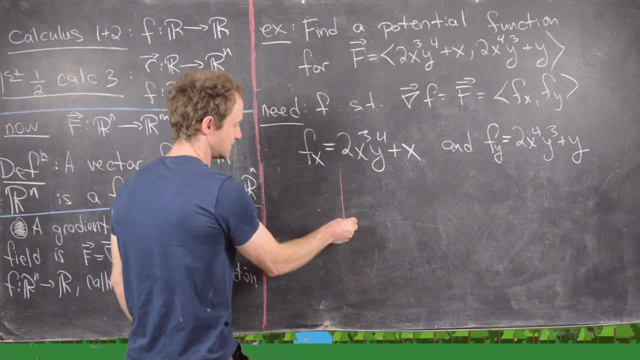 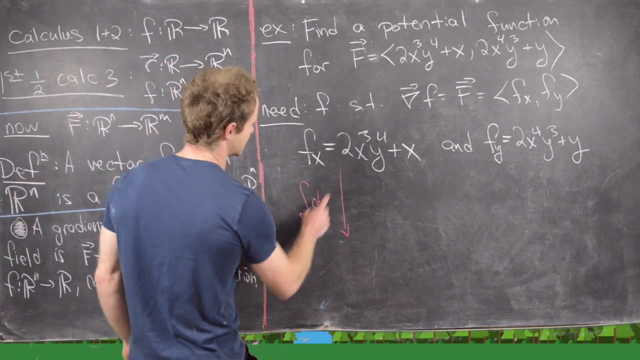 the antiderivative of this with respect to x. So I'll write that in the following way: So antiderivative with respect to x. so that's going to give us the following: So notice that will give us one half x to the fourth. 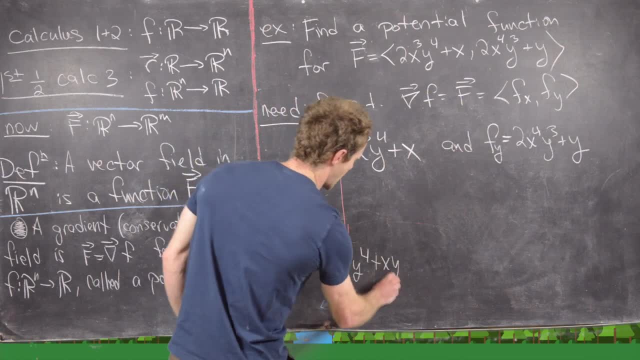 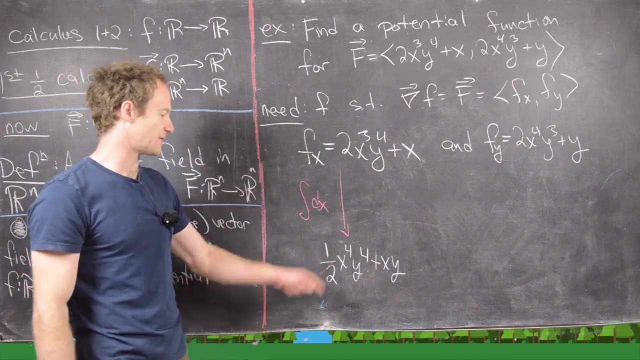 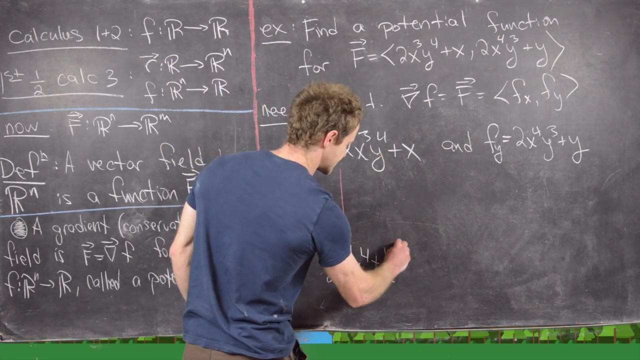 y to the fourth plus xy. So let's talk through this part. So notice, we're going to increase this exponent by one divide by the new exponent. two divided by four is obviously a half, and then one half x squared. Okay, so let's talk. 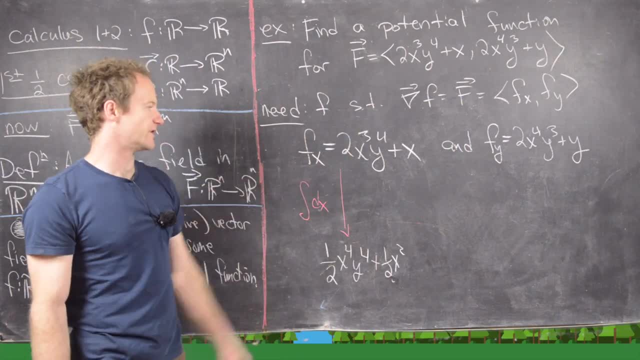 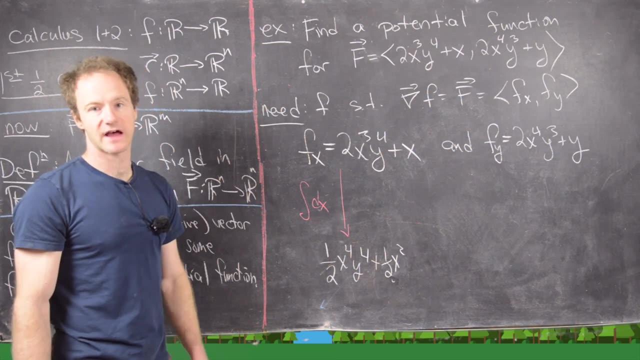 through this. So we raise the exponent by one, that's going to be a four. we divide by that new exponent: two divided by four is one over two, and then the antiderivative of x is obviously one half x squared. but I'm missing. 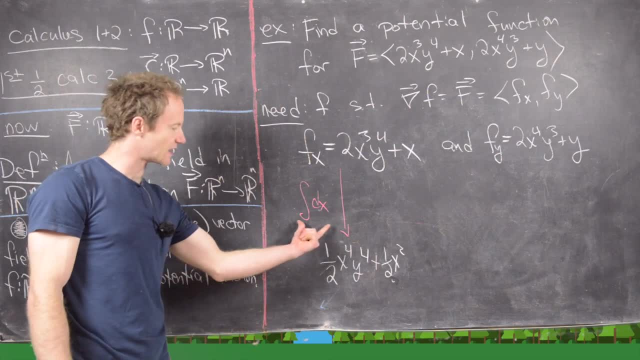 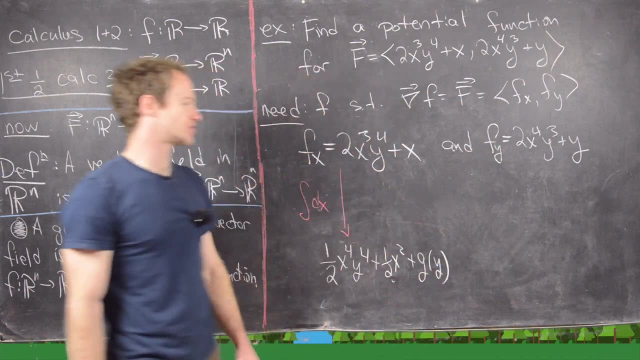 one thing: I'm missing my constant. But if I'm taking a constant with respect to an x integral, that can actually be a function of y, So I'll just write that as g of y. Okay, so now what I want to do. 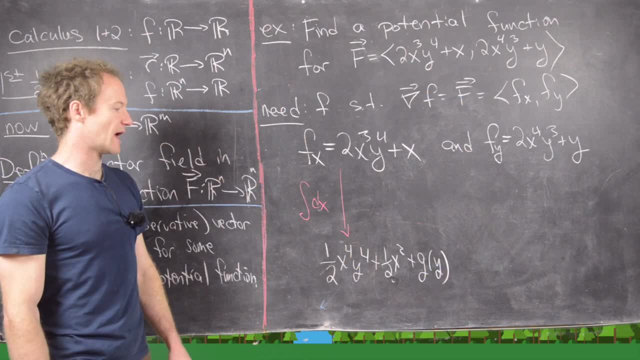 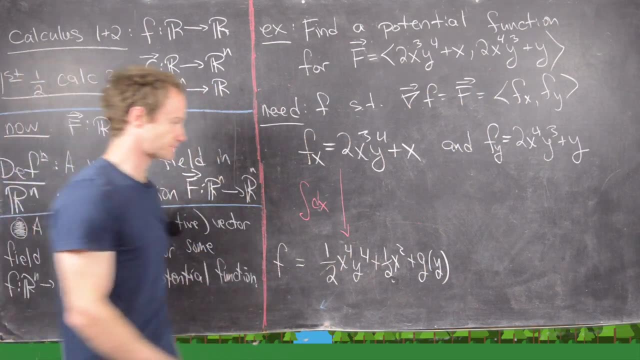 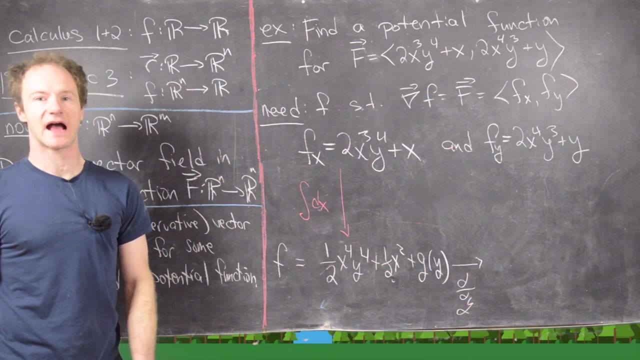 is: take the partial of this with respect to y. So notice, this is playing the role of f in this case. So if we take the partial of this with respect to y, that should match with that guy up there. So let's see what we get when we 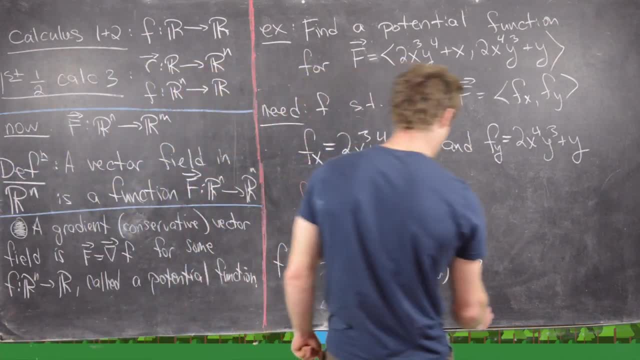 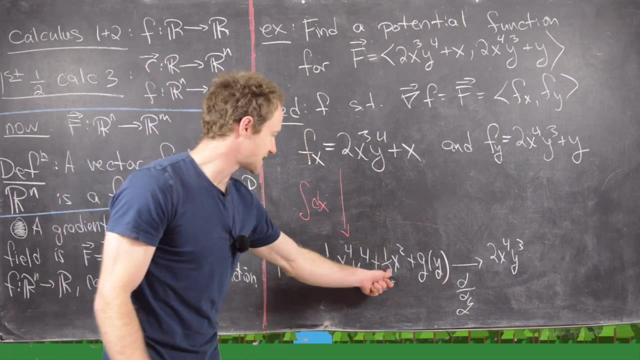 take the partial of this with respect to y. So notice that's going to give us two x to the fourth y cubed for this first term. That's going to give us zero for this second term, because that's just a function of x. 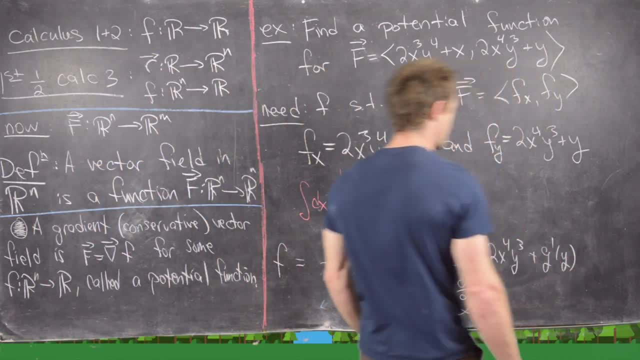 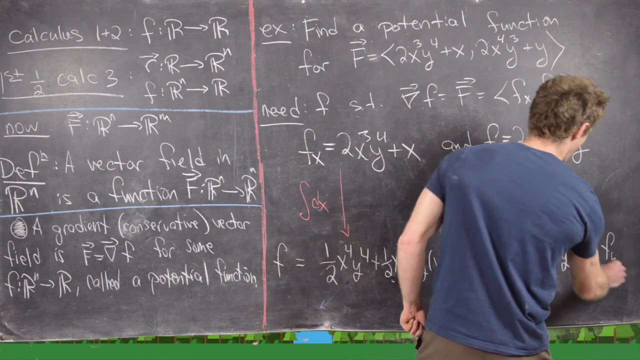 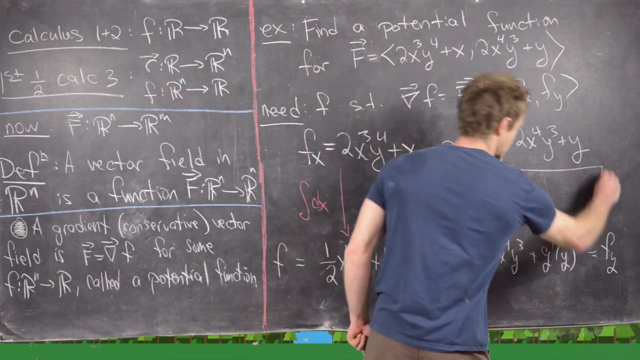 And then that's going to give us g prime of y for our third term. Okay, So now this should be equal to f sub y. Now what we do is we compare these two and notice, comparing these two, we've got this term and this term, which are the same. 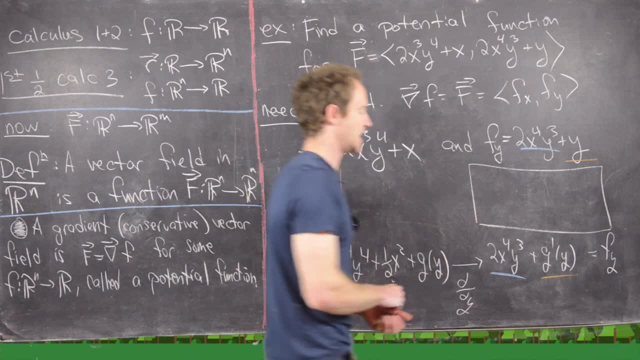 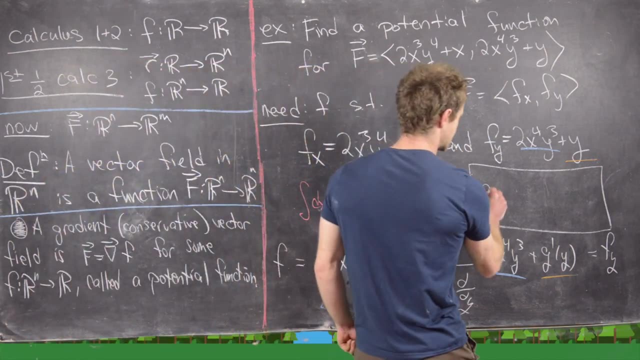 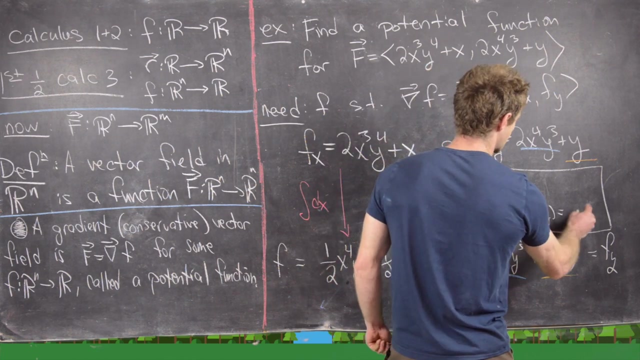 and then we've got one term left over, which, in the bottom equation, is g- prime of y, and the top equation is y. So what that tells us is that g prime of y needs to be equal to y. In other words, g of y is equal to. 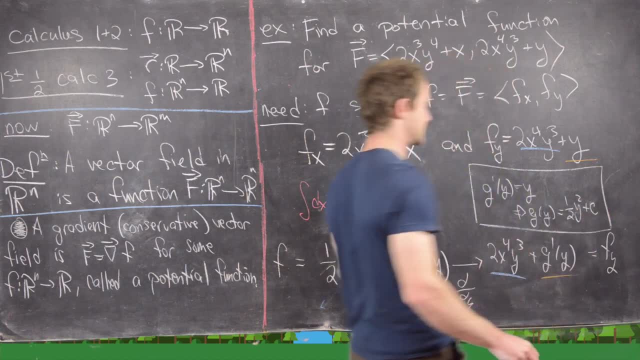 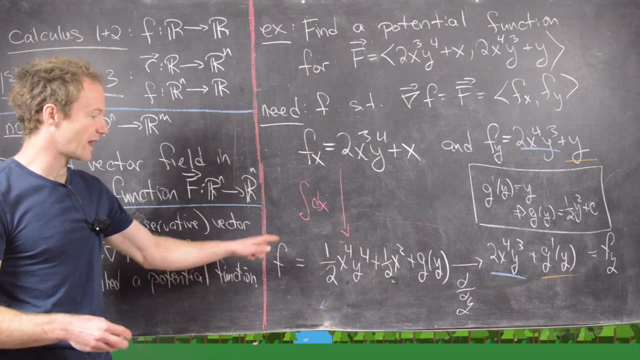 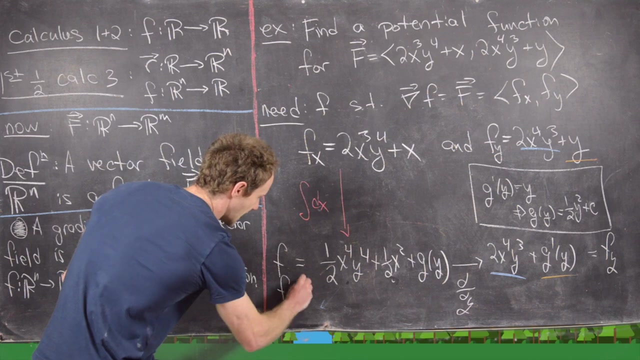 one half y squared plus a constant, And this is an actual constant, not a constant with respect to x or anything like that. Okay, So now what we can do is we can put this value of g into this function, and that will give us our potential function. 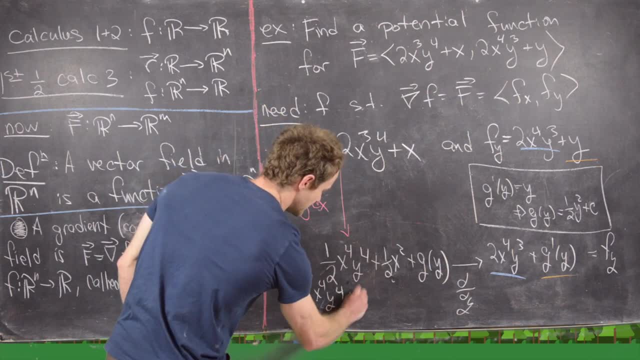 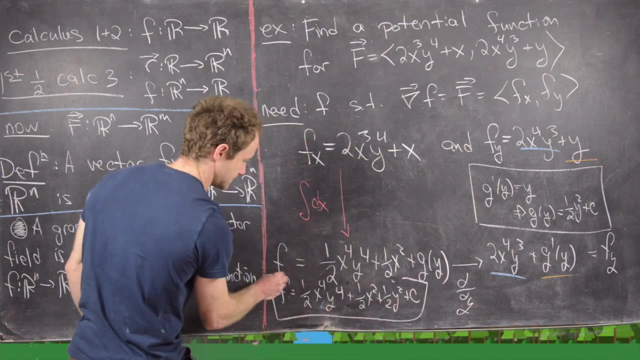 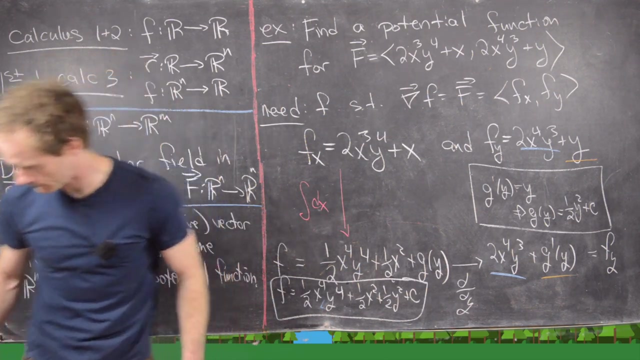 So we have one half x to the fourth, y to the fourth plus one half x squared plus one half y squared plus a constant, And that is the final answer. Okay, We'll do one more example. Okay, For our final example, we want to. 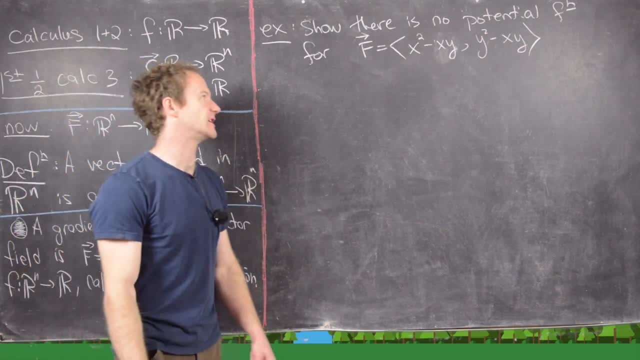 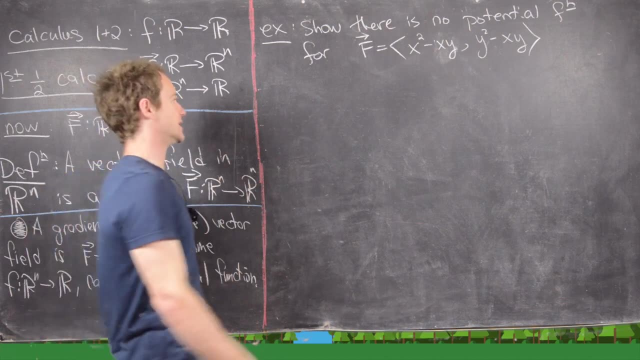 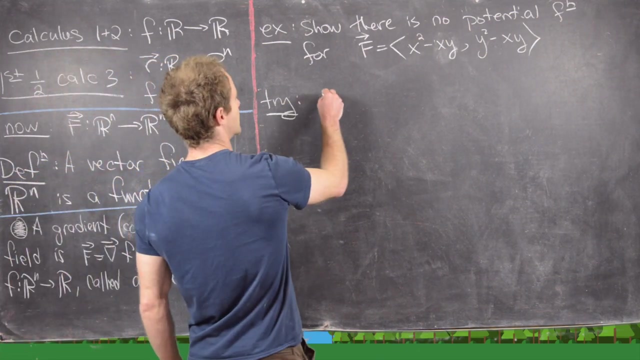 show that there is no potential function for this vector, field f, given by x squared minus xy and y squared minus xy in each component. So let's do this by trying to find a potential function and then failing. So we want to find a function, so 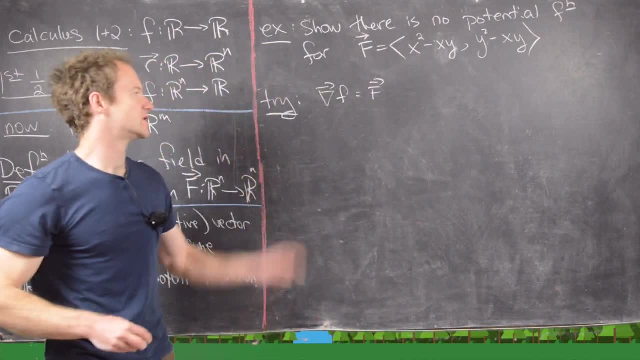 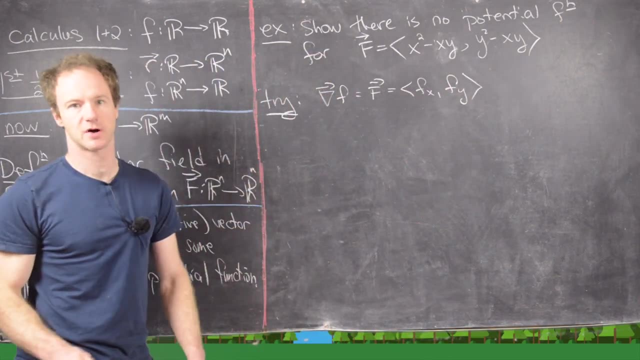 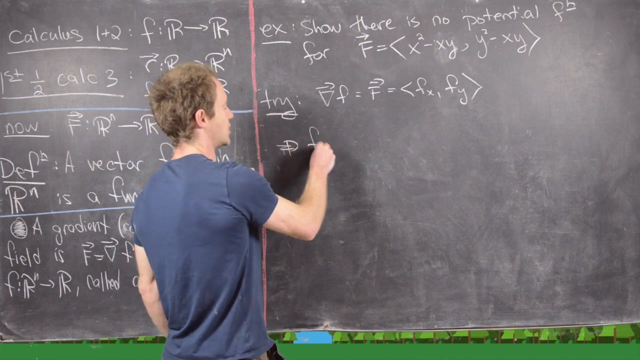 that when we take its gradient, we get f. So in other words, the partial with respect to x needs to be the first component and the partial with respect to y needs to be that second component. So what this is going to tell us is that the partial with 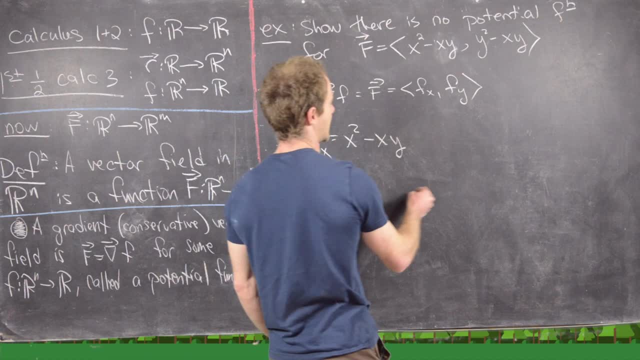 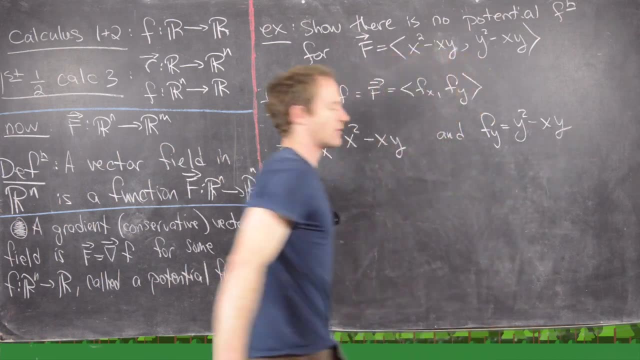 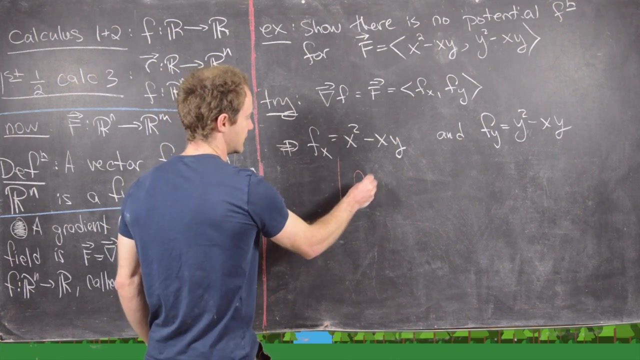 respect to x is x squared minus xy, and the partial with respect to y is y squared minus xy. Now we're going to play the same game that we did in the previous example, So I'm going to go ahead and take the anti-derivative. 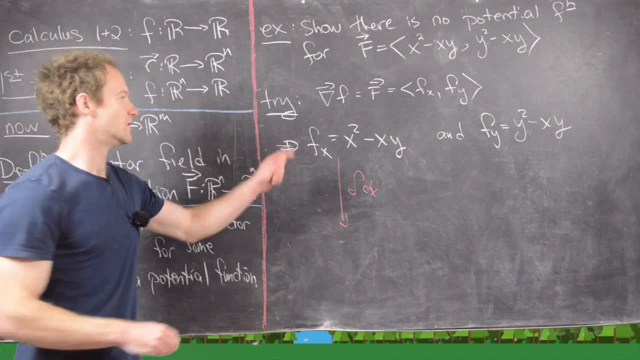 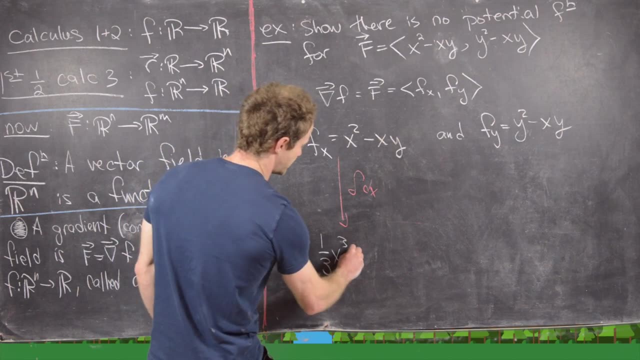 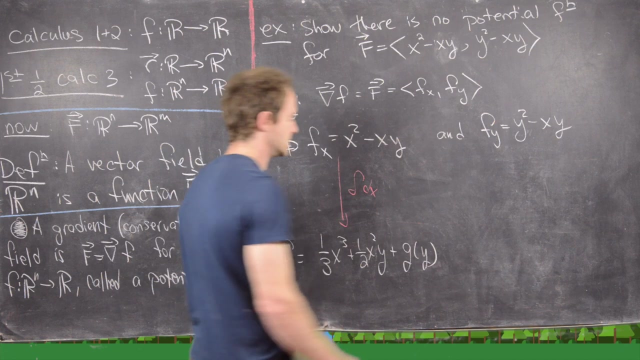 with respect to x on this side. So notice, that's going to give me: f equals one third x cubed plus one half x squared y plus g of y. So my constant of integration here is a function of y. Great, Now I'm going to take the partial. 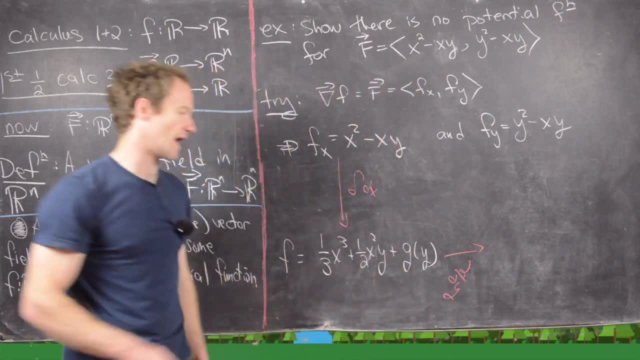 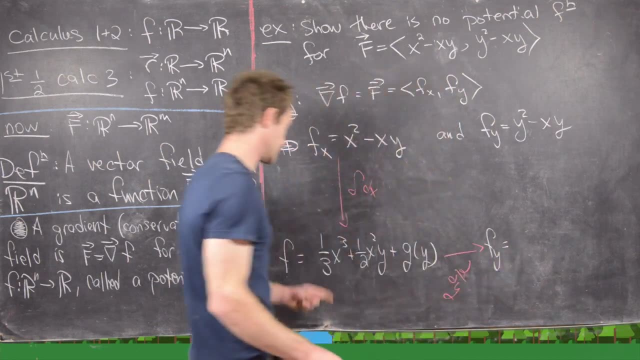 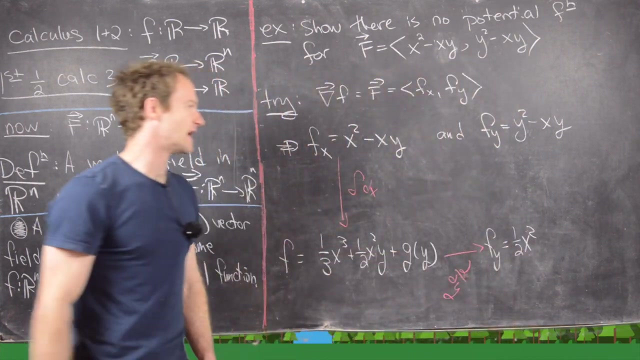 derivative of this with respect to y. So that's going to create f sub y equals. so that's going to give me zero, That's going to give me a half x squared, and then that's going to give me g prime of y.